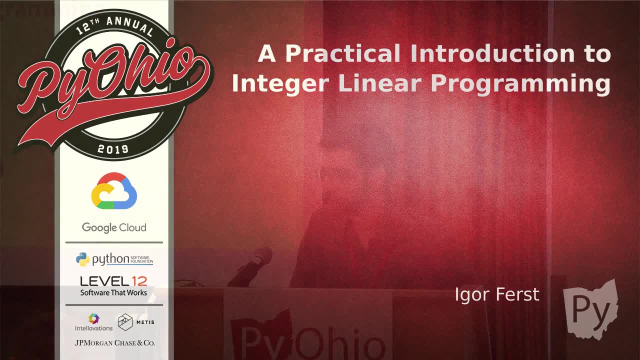 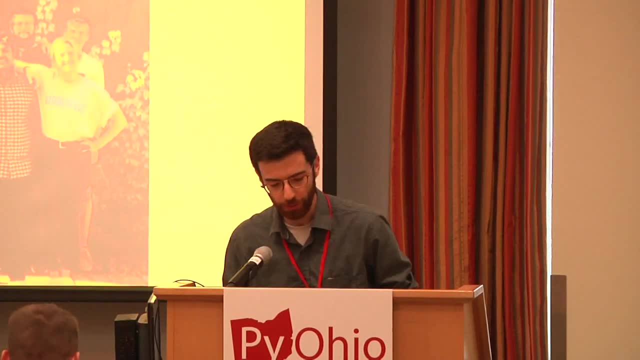 Great, All right, Let's get started. Welcome to a practical introduction to integer linear programming. I'm Igor First. I live here in Columbus. I'm co-founder and CTO of Mobikit. We are a very early stage venture-backed software startup. We are building tools to empower the use of data in mobility. 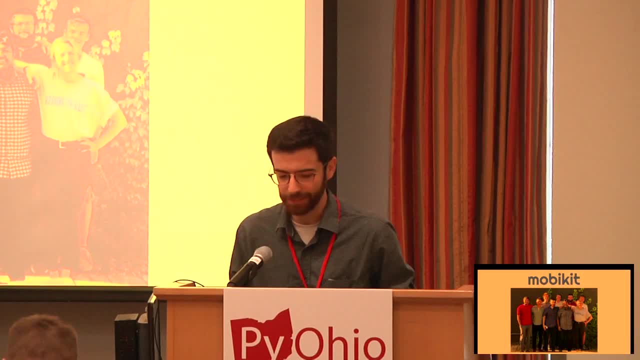 And I'm here to talk to you about integer linear programming because, to my delight, this is actually something that came up in some work that we were doing earlier this year for a customer, and I thought some other folks might be interested in learning a little bit more about it. 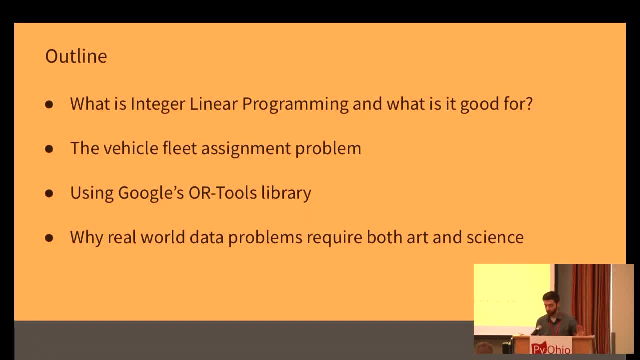 So here's what the next half hour is going to look like. We'll start by talking about what is integer linear programming. I'm going to call it ILP, usually to you know, say fewer syllables. I'm going to talk about what it is and what kind of problems it's good for. I'm going to talk about the vehicle fleet assignment problem. 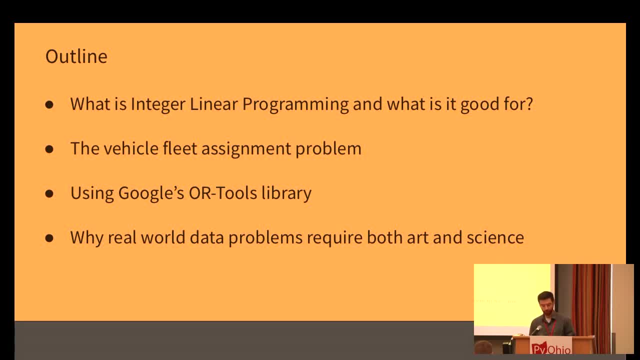 which is the particular problem that we're going to talk about today. I'm going to show you guys how to phrase it as an ILP problem and then use Google's OR tools library to solve it, which is an open source Python library, And then, time permitting, at the end I'll spend just a couple of minutes talking about how our problem and ILP in general are a great illustration of the fact that solving real-world data problems is as much art as it is science. 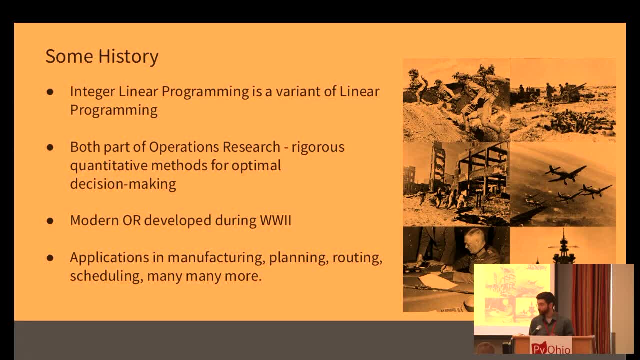 So if that sounds good, let's get started with just a little bit of information. Thank you, So we're going to start with the literature of history. Integer linear programming is a variant of linear programming. There was a really good talk on linear programming yesterday. 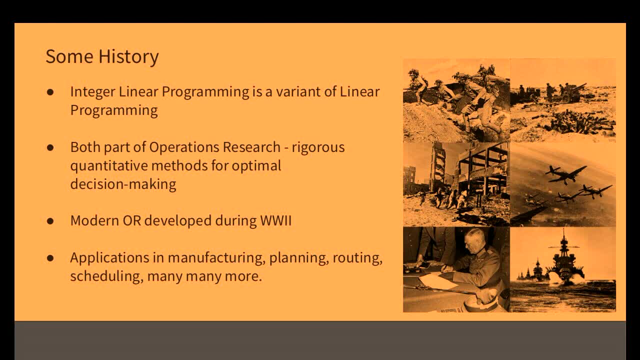 If you guys went to that talk and you're also here, rest assured you will see lots of new things. so don't worry about that. But both of these fields are actually part of operations research, which you can define kind of broadly as the study of rigorous quantitative methods for optimal decision making. 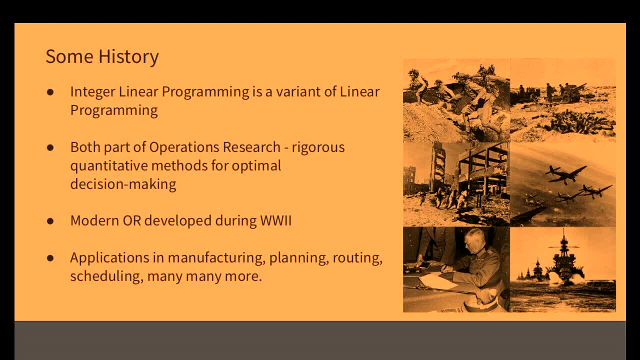 And modern operations. research developed during World War II, when people had a lot of very high-stakes decision making making they needed to do, and they wanted to do it optimally. So people had to answer questions like how to route supply lines through Europe or like how 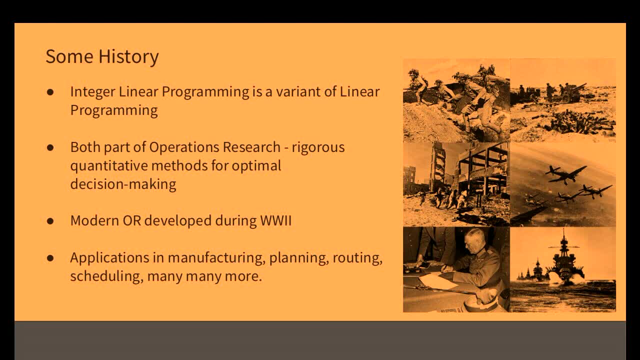 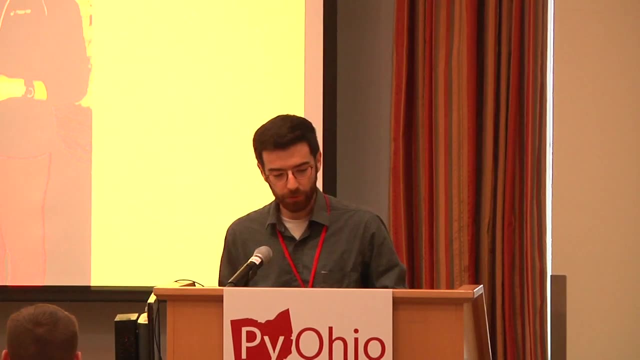 to optimally select bombing targets and things like that. and they developed a lot of extremely useful quantitative methods to answer those kinds of questions and in the decades after World War II there were applications in manufacturing, planning, routing, scheduling across many, many, many different domains. A little bit of personal history I learned about. 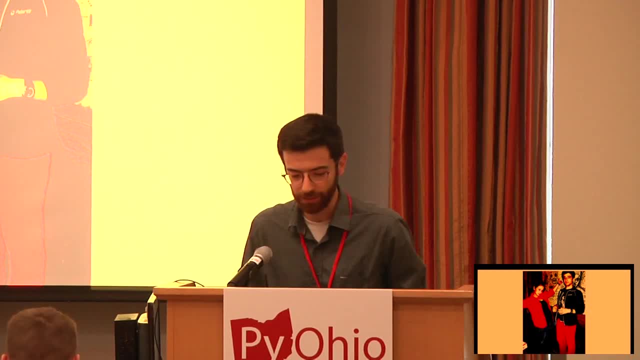 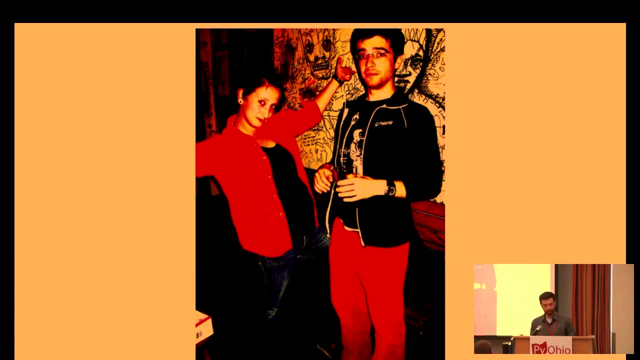 operations research from my wife, Rachel, that's us in grad school during our SALAD days. Rachel was actually in a graduate program in operations research and I was in a different program, but she taught me a whole lot about it and for that I'm very grateful. and Rachel will continue making some appearances. 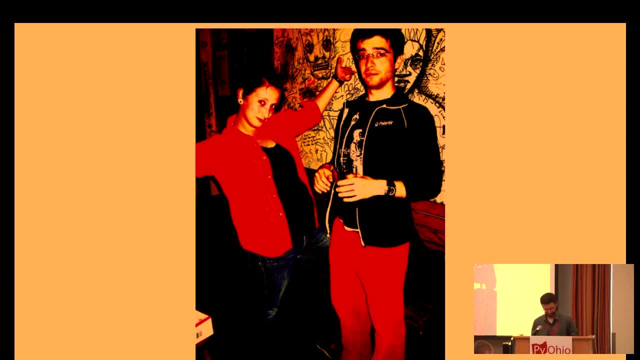 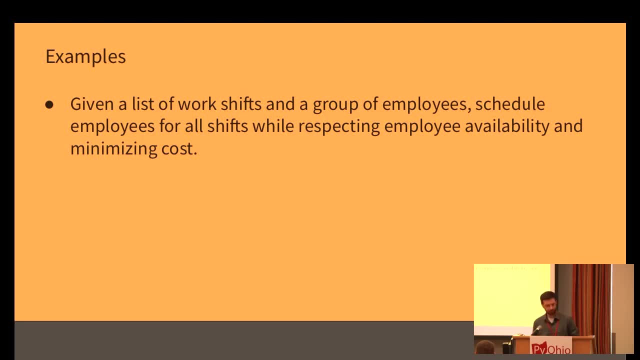 throughout this talk to help us along our ILP journey. Okay, great. so ILP, what kind of problems can you solve with it? And before I give you kind of a general statement, let me just give you some examples, some concrete examples that I hope will motivate things a little bit. 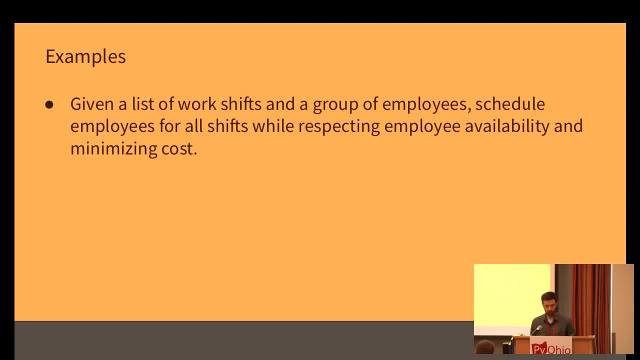 So here's a great problem. it's the employee shift assignment problem, kind of a classic ILP problem. So here you have a list of work shifts, you're an employer, you have a list of work shifts, you have a group of employees you want to. 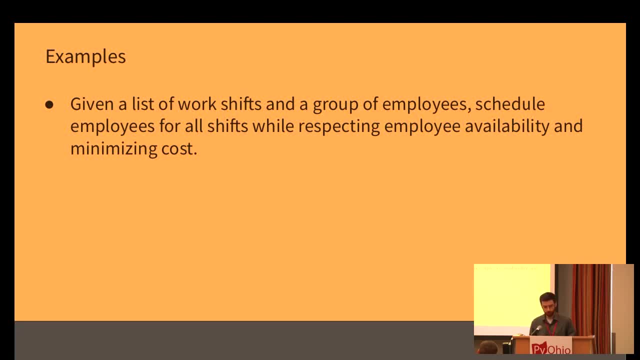 schedule employees for all the shifts while respecting employee availability and, of course, minimizing cost. you're the business owner and you're hard-nosed and you want to minimize cost. Here's another example. this is generally called the facility location problem. So I imagine you want. 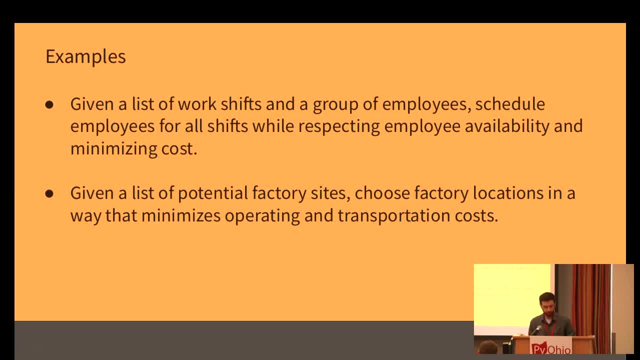 to build some factories, to make some widget, and you have a large list of potential factory sites. You need to select some subset of those sites to actually build those factories and you want to choose those sites in a way that minimizes the operating cost for the factories but also minimizes the 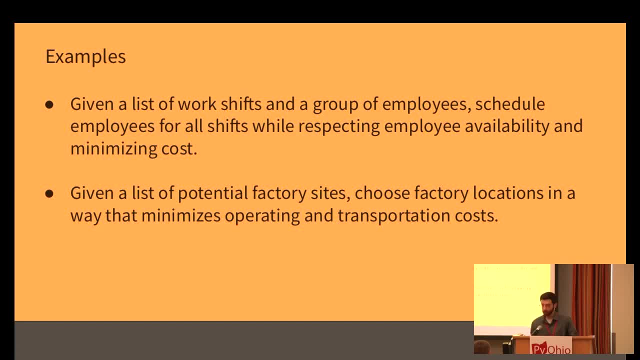 transportation cost for the widgets that you're gonna be sending out of these factories. Another very classic ILP problem. Here's another good one. we'll actually dig pretty deep into this one. This is the vehicle fleet assignment problem. You have a list of. you have a fleet of. 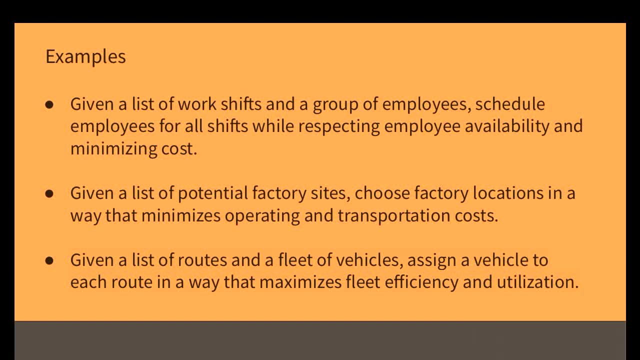 vehicles and you have a bunch of routes that need those vehicles to drive. So you want to assign a vehicle to each route in a way that maximizes fleet efficiency and utilization. So you can think of these routes, as you know, like transporting people. So imagine a route. 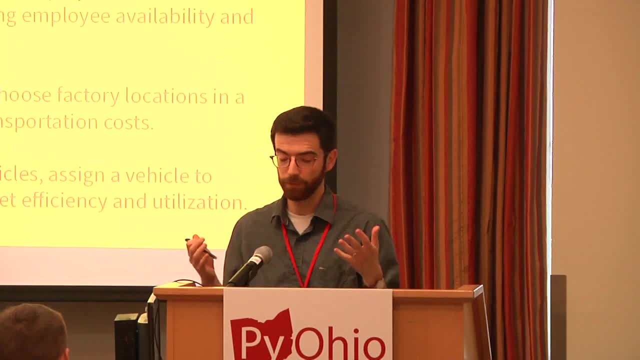 is just a group of people that has to go from point A to point B, and you have a fleet of vehicles. You want to figure out which vehicles to use for what route in a way that is most efficient- Great. So the thing that all these problems have in common is that kind of 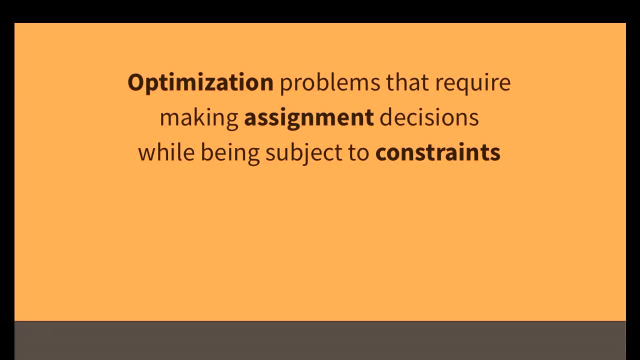 broadly speaking, they're optimization problems that require making assignment decisions while being subject to constraints. So you're making assignment decisions, you're assigning employees to shifts, through vehicles, to routes, and there are constraints around which assignments you may or you may not make. And you're, and you have some optimization, you're trying to. 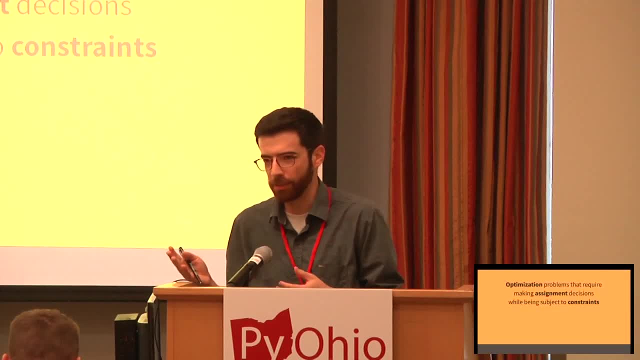 do, in the sense of you have a definition of what's a good assignment and what's a bad assignment and you want the best possible assignment according to the task funnel. You want as many options according to the strategy. So feature design is one step away from platform design. It's theb deriving of your시는 requirements andengineч на. 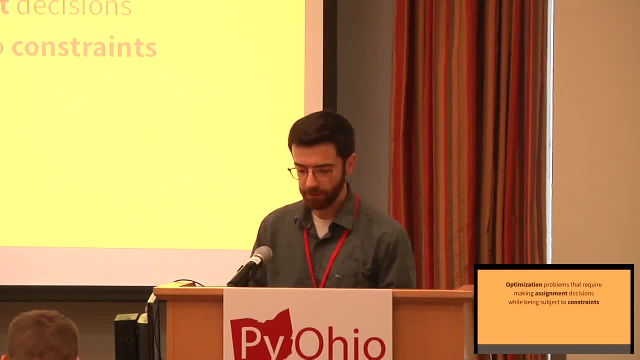 some. you know some metric. So broadly speaking, these are the kinds of problems that ILP is good for. But of course there's a little bit of a catch: You can only use ILP if you can represent your problem in a particular mathematical. 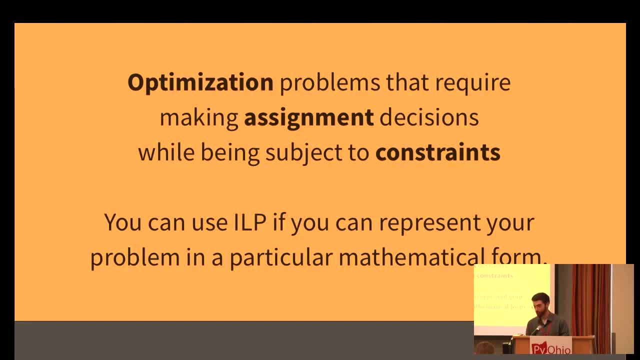 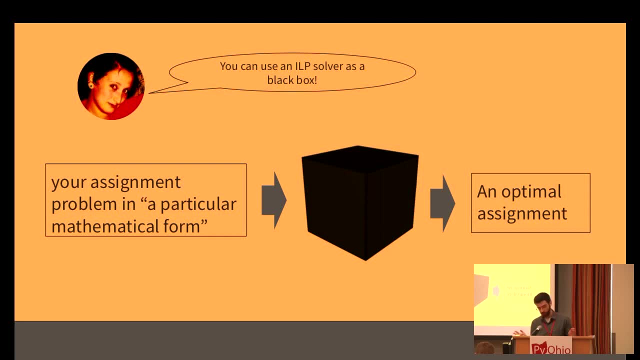 form, And I'm going to get to the details of what that particular mathematical form is. But before I do that, I'll just say that if you can represent your assignment problem in this particular mathematical form, that's pretty good, because you can use an ILP solver. 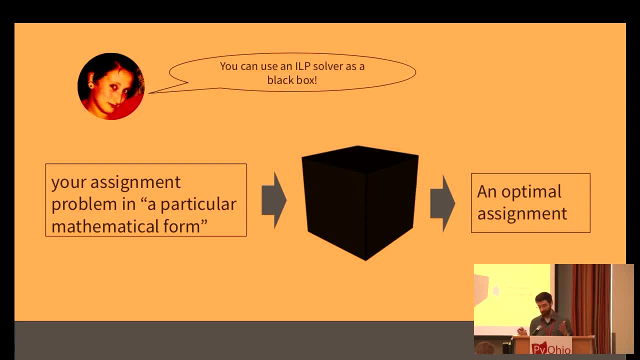 in a totally black box fashion. There are ILP, solvers, open source and proprietary. you kind of pull off the shelf, you put your problem in the special form, you put it on the solver and the solver will give you an optimal assignment, an assignment that is provably optimal, you know, with respect to 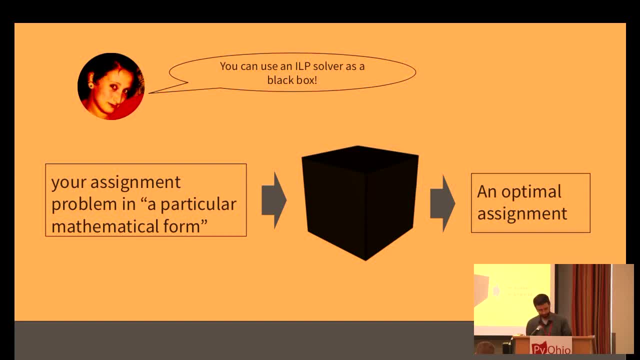 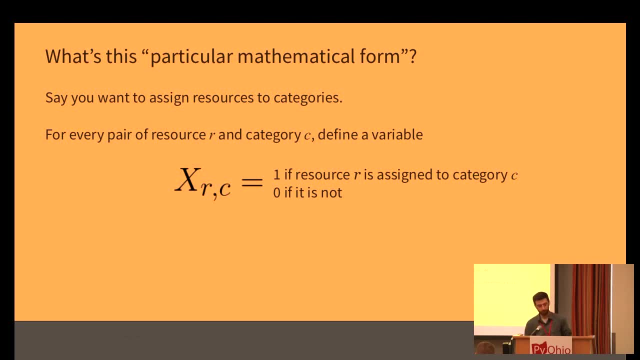 the problem that you had fed it, which is pretty great. Okay, So what is this particular mathematical form? Let's talk about it. I'm going to tell you what it is and I'm going to use the employee shift Scheduling problem to kind of help define this. 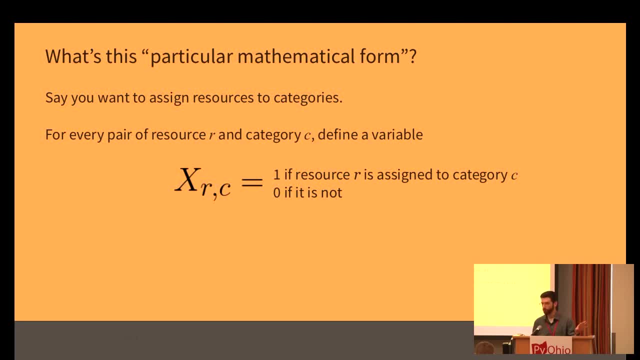 And then after that we're going to actually put the, we're going to go back to the vehicle fleet assignment problem and we're going to work through putting it into this particular mathematical form. Okay, But what is it? So let's say you have an assignment problem or you're assigning resources to categories. 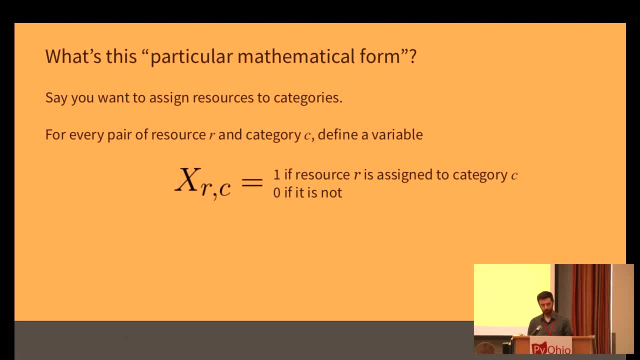 just fairly generally speaking. So you start, in order to put it in this particular mathematical form, you start by defining a variable XRC for every pair of resources- I'm sorry, for every pair Of resource R and category C for every possible pair. 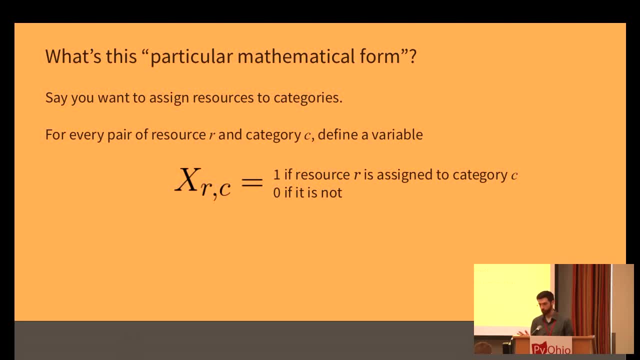 And these variables are allowed to take only two values- zero or one. And if their value is one, that means you're assigning resource R to category C, and if value is zero it means you're not. So, for example, with the employee shift assignment problem, there's an XRC for every combination. 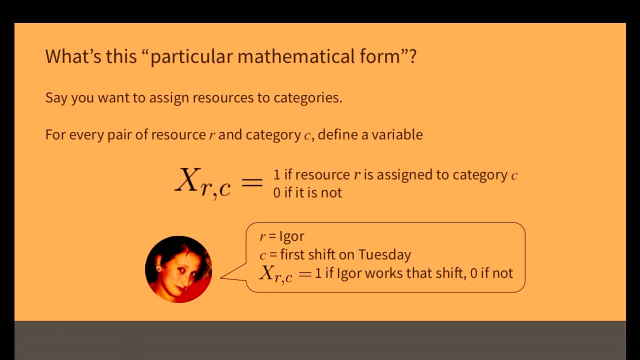 of employee and shift. So, for example, there's employee Igor a shift, that's first shift on Tuesday, and then there's a variable XRC That corresponds to that pair. Its value is one if we're going to have Igor work that shift. its value is zero. otherwise, 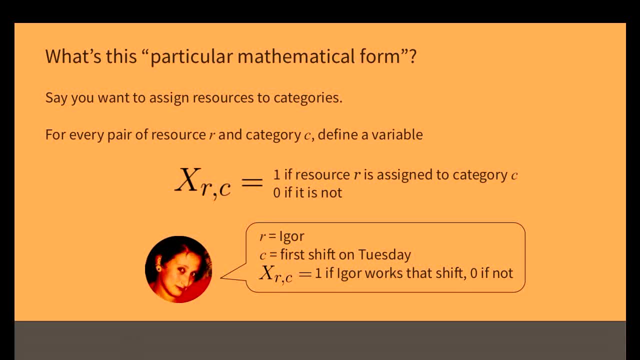 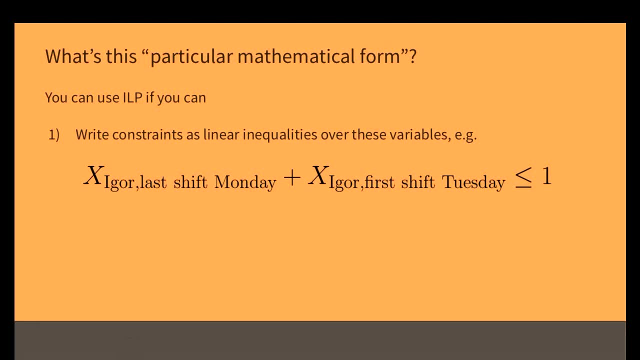 Great. So you define all these variables And now you get to use ILP if two things are true. if there are two, if there's two conditions hold. Condition number one is all the constraints in your problem, are all the constraints around. 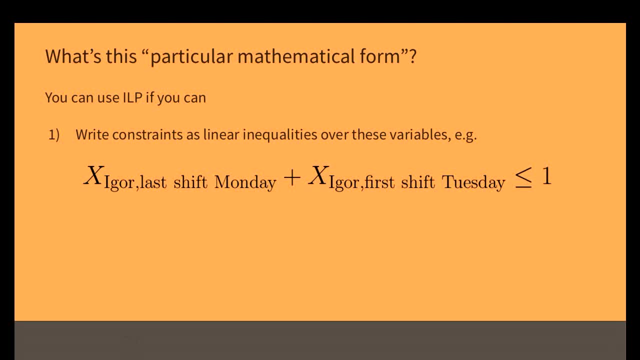 the assignments that you're allowed to make, you have to be able to write them as linear inequalities over these variables. So, for example, If one of our constraints is we don't want to make people close the store one night and then immediately open it the next morning, you would write that constraint like this: 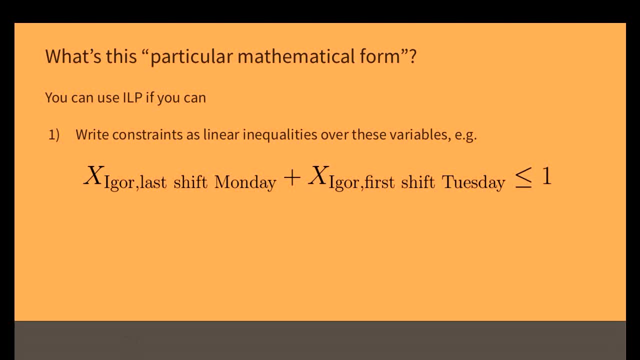 So X Igor last shift Monday plus X Igor first shift Tuesday, is the most one, And this represents that constraint accurately, because these are all zero, one valued variables. So what this constraint is saying, both of these assignments cannot be true. We're not going to allow that. 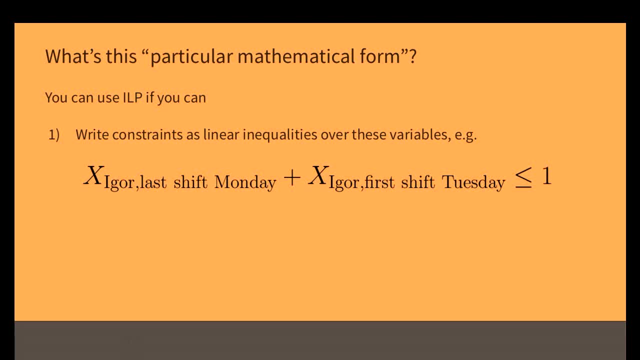 So you have to be able to write every single constraint as a linear inequality. The second condition is the function that you're trying to optimize. either minimize or maximize, either works the function you're trying to optimize. you have to be able to. 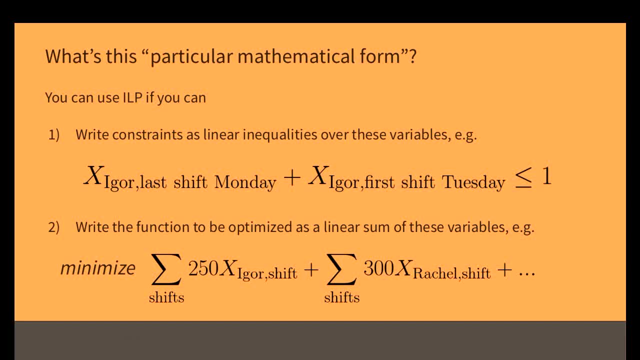 write it as a linear sum of these variables. So for example here in the employee shift assignment problem, let's say we want to minimize cost. then we can say, okay, write out this very, very large sum that just takes all these. 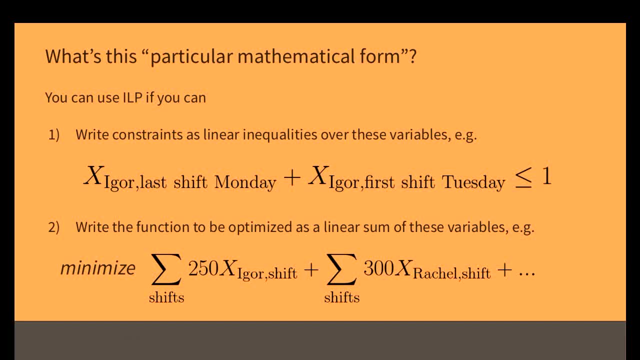 variables, multiplies them by the cost of the assignment, And then you can write it as a linear sum. So for example here in the employee shift assignment problem, let's say we want to minimize cost, So we can write out the cost of assigning an employee to a shift and then add them. 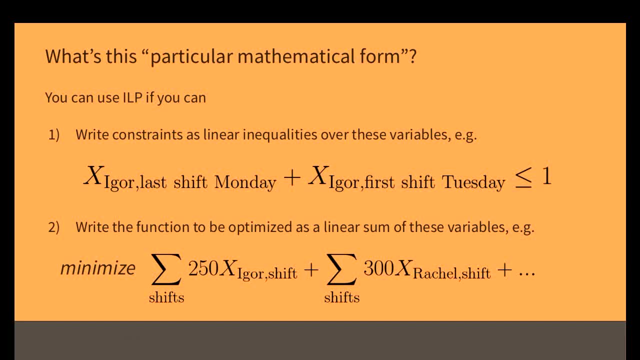 all up. And so, because these are all zero one variables, we know that taking this sum over all possible employees, that's just going to be the total cost of the employees that you assign to all your shifts, And so you can write it as a linear sum and then you can just say: I just want to minimize. 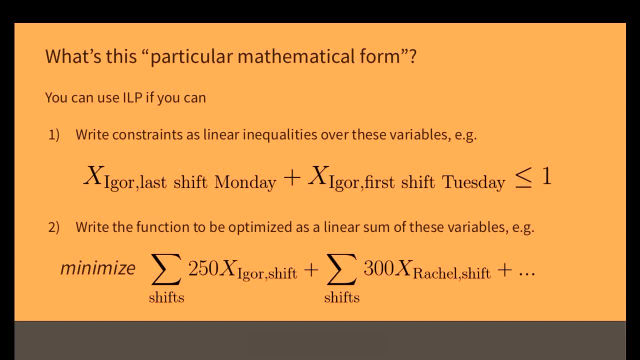 this. I just want to minimize this total quantity. So if both of these conditions hold, then congratulations. This is the mathematical formula, Thank you, Thank you. So you have the form required to be able to use an ILP solver, And so you can just put your problem in this form, feed it into the solver, get an assignment. 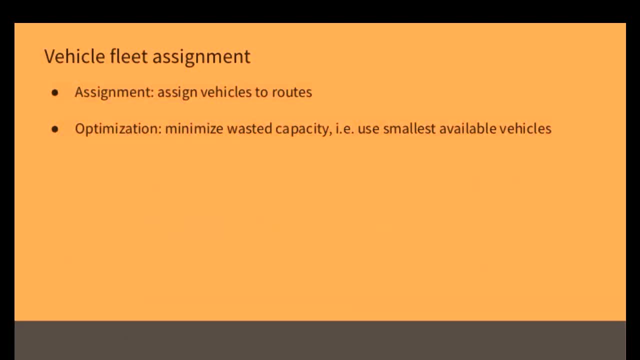 back and link back in quiet satisfaction, Great. So that was kind of a high-level example. so now I want to go deeper with the vehicle fleet assignment problem, And this is the problem that we had to solve. So I'm going to give you kind of a simplified version of the problem that we ended up solving. 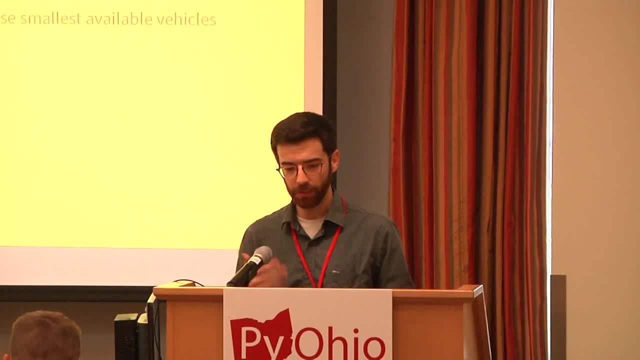 from one of our clients And I'm going to show you guys exactly how to encode it into this form. And then I have a little notebook where we actually take that representation, we fit it to Solver and we get a solution. It's great. 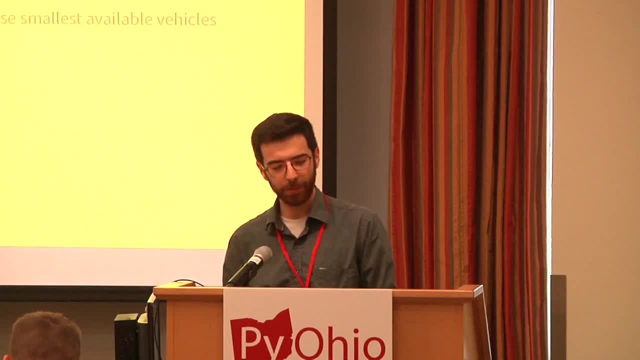 All right. So vehicle fleet assignment: In this assignment we're assigning vehicles to routes And again, a route is just a group of people that needs to be transported, So a group of people fixed size going from point A to point B. 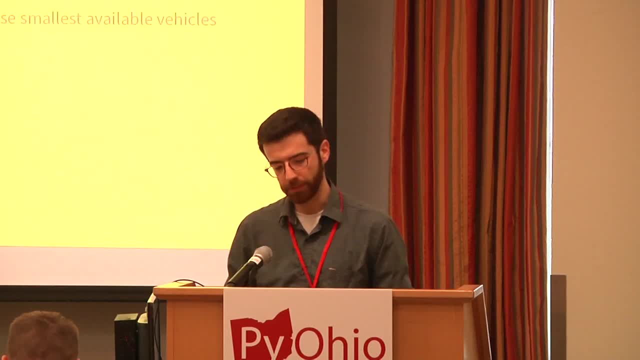 The optimization we wanted to make is: we want to minimize wasted capacity, So we want to use the smallest available vehicles for these routes. You know, if a route only has two people, don't send a very large bus to transport those two people. 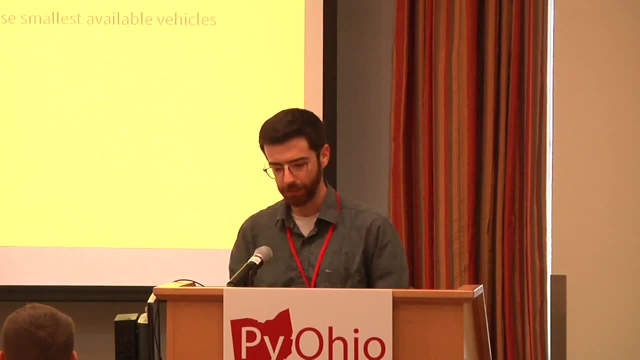 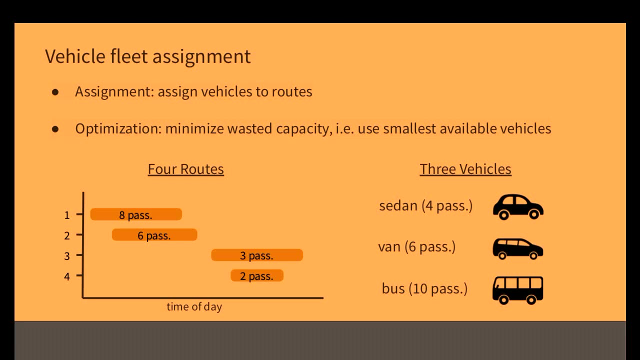 Because it's inefficient and you know you waste fuel that way if you send a vehicle that's too big. Okay, So to be concrete, let's just imagine this very small, simple instance of the vehicle fleet assignment problem. So we have four routes. 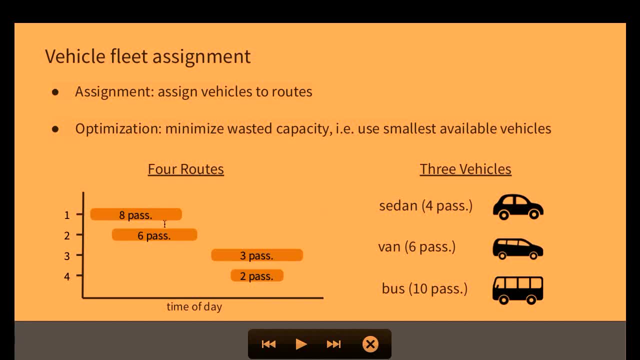 This is kind of a Gantt-like view of of the routes with respect to the time of day. So we have these two routes in the morning With eight and six passengers and then a couple routes in the afternoon with three and two passengers. 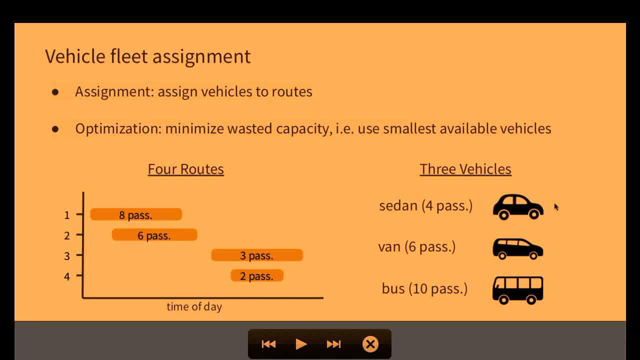 So we've got these four routes we need to service. We have three vehicles in our fleet: Sedan that seats four, not including the driver, A van that seats six and a bus that seats ten. So how do you assign these vehicles to these routes? 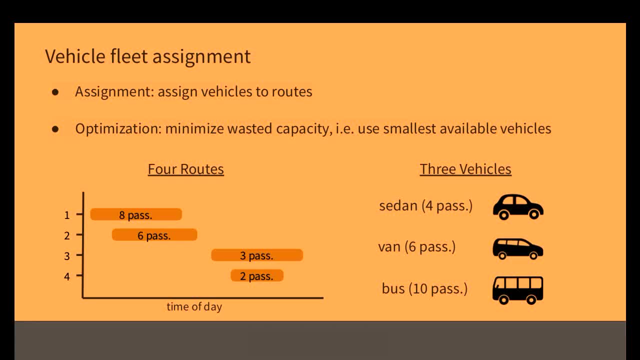 We're gonna write up all of our constraints. We're gonna figure out where our constraints are, write them all up and then feed that problem to our solver. So let's think about the constraints. One very reasonable constraint is: you wanna assign a 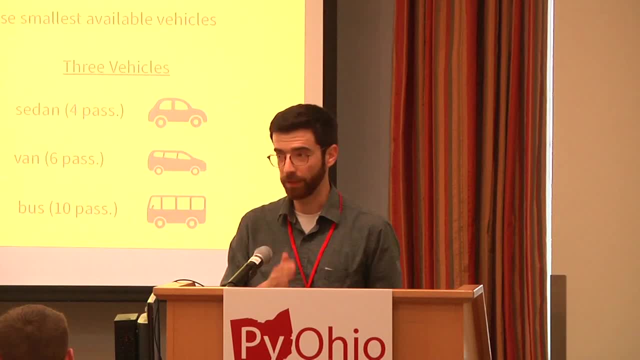 vehicle to every route. You don't wanna leave anybody hanging. you wanna make sure that every route gets a vehicle And, for the sake of simplicity, let's just say that we wanna assign exactly one vehicle to each route. One vehicle just to serve a route. 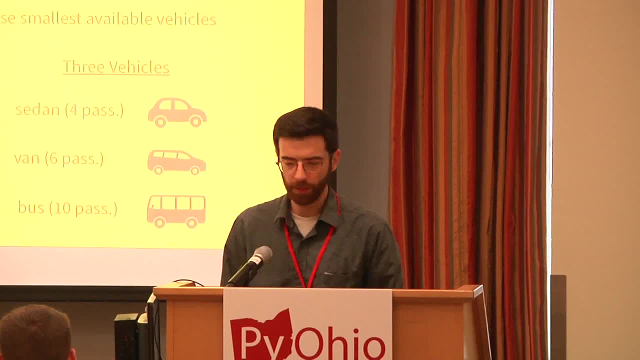 OK. So that's the first kind of constraint that we wanna apply And we're gonna. I'm gonna call those coverage constraints. We wanna make sure that all of our routes are covered, OK. The second constraint is, obviously you can't use any. 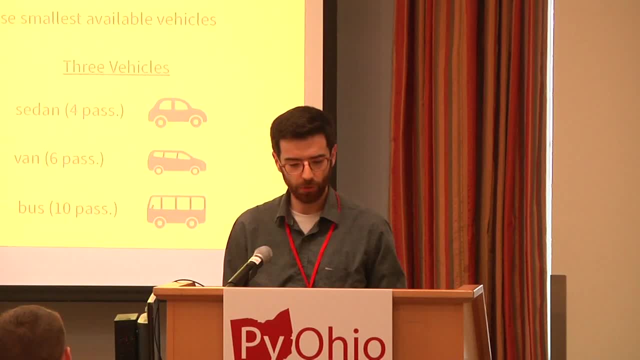 vehicle for any route. Some vehicles are too small for certain routes. So this is the second type of constraint. I'm gonna call these capacity constraints. You have to make sure that the vehicle that you assign has sufficient capacity to handle the route. The third type of constraint just says: all right if 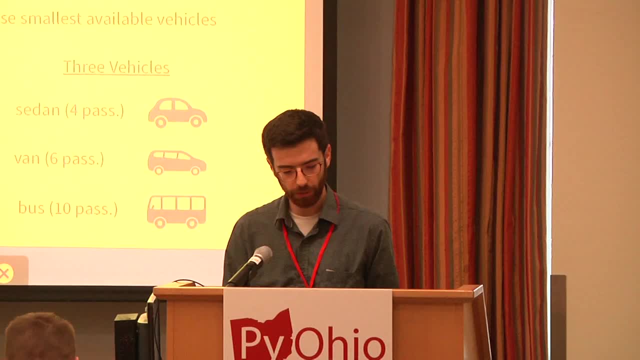 we have two routes that overlap in time, like these two here or these two here, we can't use the same vehicle for both, Because that vehicle cannot be in two places at the same time. And so this last set of constraints overlap constraints is what I'm gonna call. them just says: 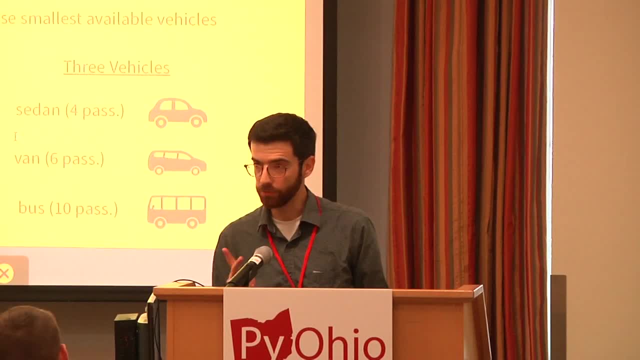 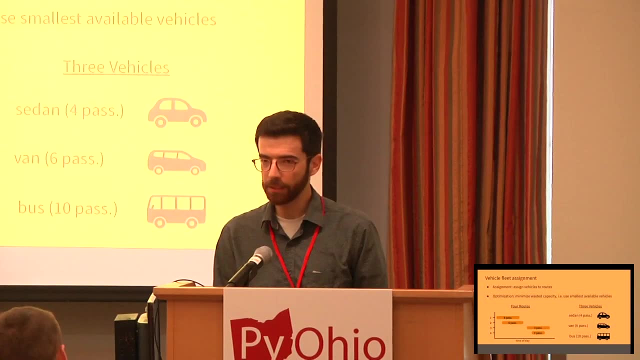 you can't assign a vehicle to two routes if those two routes overlap in time. So three types of constraints. Now I'm gonna stop there, because at this point this problem is like realistic enough. Now, in practice, you can imagine lots of other types. 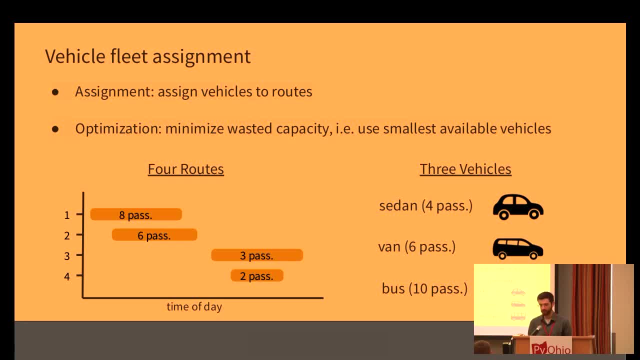 of constraints, Like maybe not every vehicle is available at any time of day, Or maybe you can't assign a vehicle to do two routes. if the two routes are very far away from each other, They're not gonna get to them in time. So all that is true. 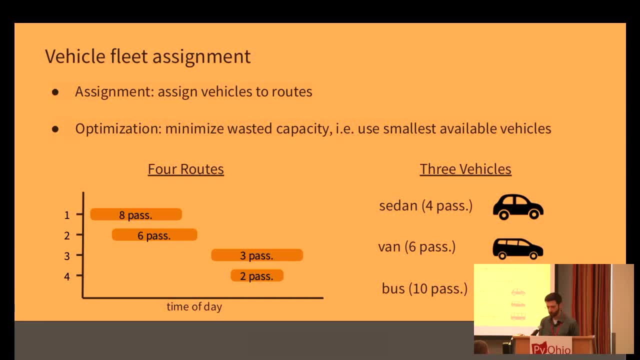 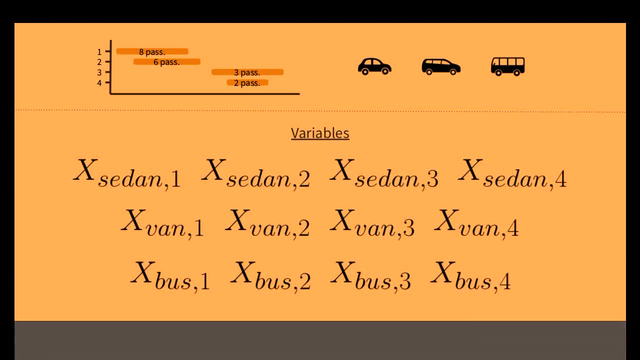 But for the sake of simplicity, let's just stop here, because this is realistic enough to move forward. OK, Great. So we have these constraints. How are we gonna write these constraints as linear inequalities? We need to do that in order to be able to. 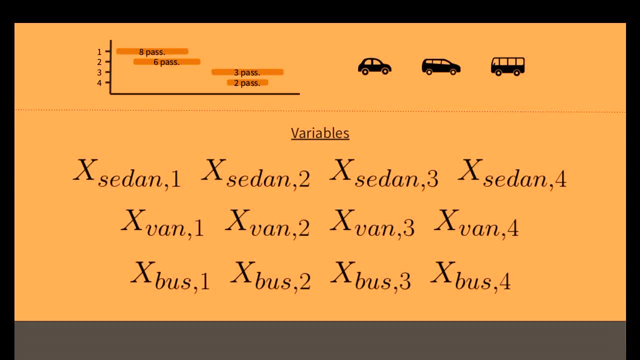 feed this problem to a solver. So first we start with our variables. So we have four routes, three vehicles, which means we have twelve variables, one for each vehicle route pair, And again, in any assignment, these variables are gonna have zero, one values. 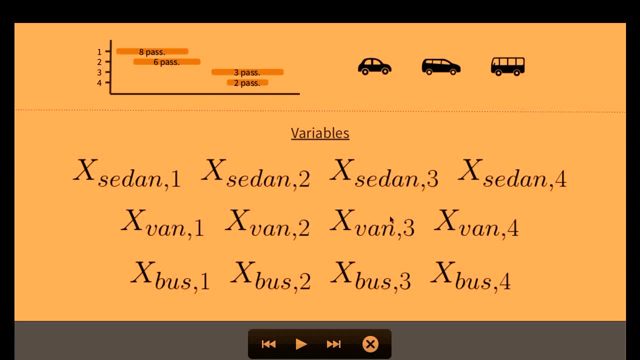 And, for example, if x van three is one, then we're gonna have zero one values. And for example, if x van three is one, then we're gonna have zero one values, And if x van three is one, that means we're gonna assign the van to. 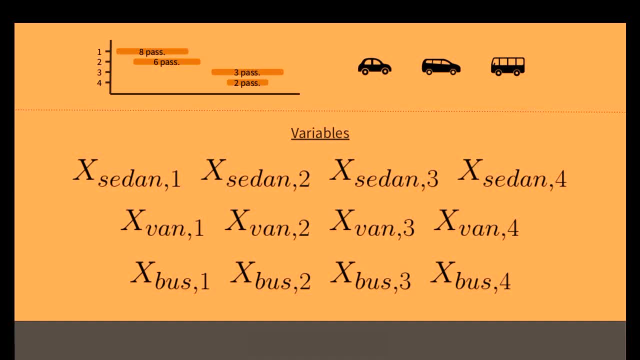 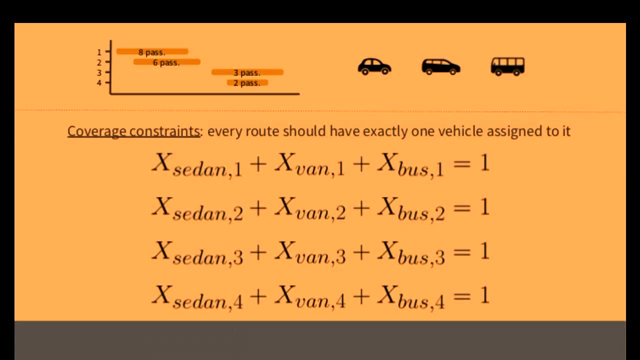 route three, And if it's zero, that means we're not. We're gonna use something else for route three. OK, Because we've got our twelve variables. So let's start capturing our constraints as linear inequalities over these variables. We'll start with the coverage constraints. 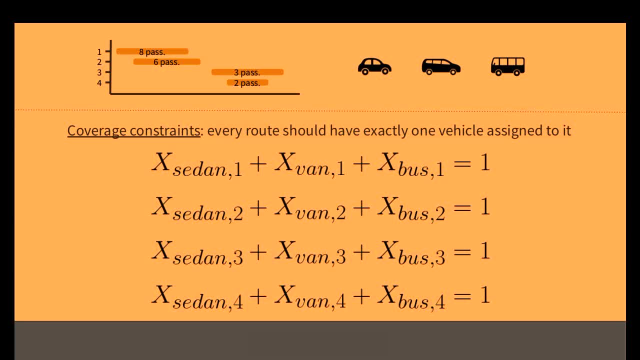 Coverage constraints say that every route should have exactly one vehicle assigned to it, And these look like this: There's one constraint for every route And the constraint says: when you add up all these x's over all the vehicles for this one particular route, it has to equal one. 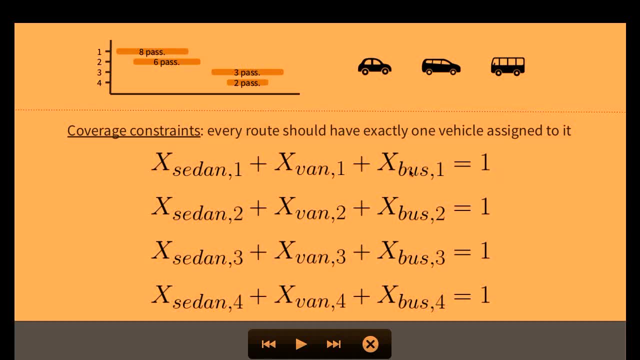 And so this does exactly what we want it to, again, because these are zero-one valued variables. So what this constraint says, for example, is: for route one, only one of these can be one. In fact, precisely one of these must be one. 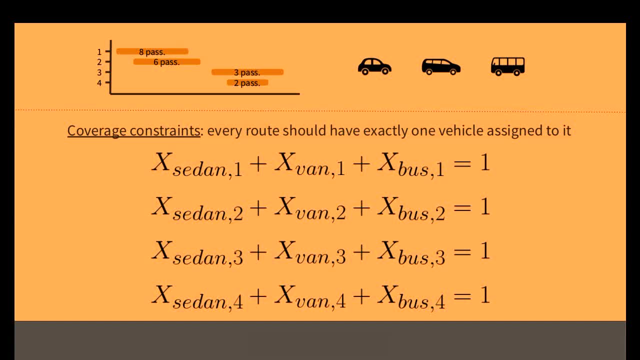 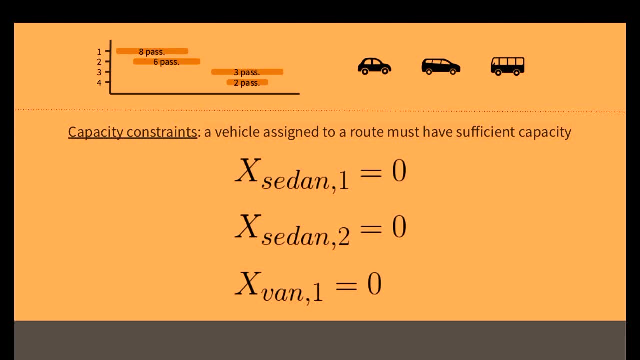 So we have one of these for every route. These are the coverage constraints, Capacity constraints: A vehicle assigned to a route must have sufficient capacity. So really, this just says we need to identify which combinations of vehicles and routes are forbidden and then just force those variables to be zero. 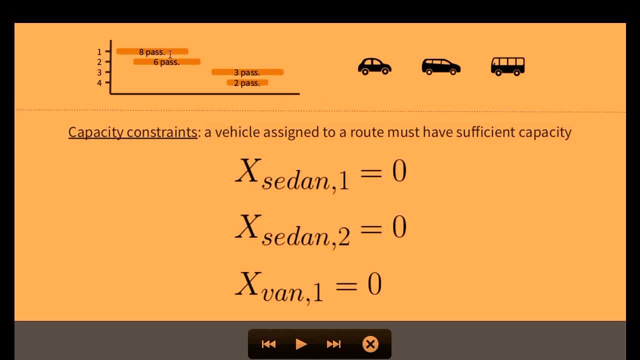 So the sedan, for example, can't serve routes one or two, It's too small, And so we're going to say in every assignment these have to be zero. Similarly, the van cannot serve route one. It's too small, so it gets one of these as well. 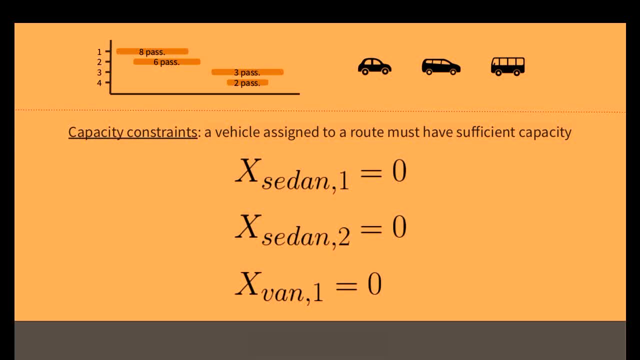 If you've been paying attention, you'll notice that I spoke in terms of linear inequalities in the very beginning, but I'm using equalities here. Of course, you can create a quality with two linear inequalities, And so that's why I'm loosely just using 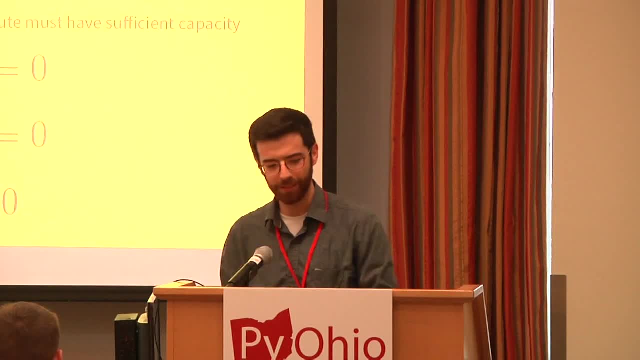 equalities all over the place. So if I want something to be equal to something else, I can say that something has to be less than or equal to that thing and also greater than or equal to that thing. So in practice, under the hood, you can give an ILP solver. 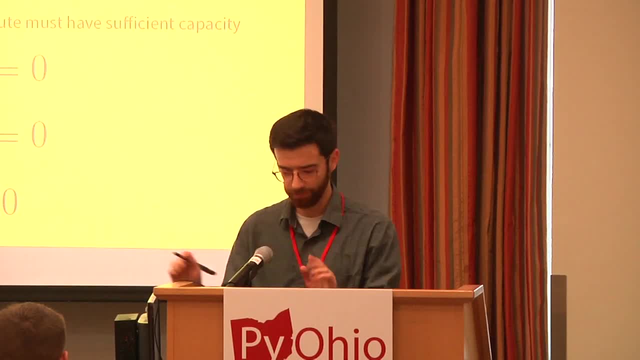 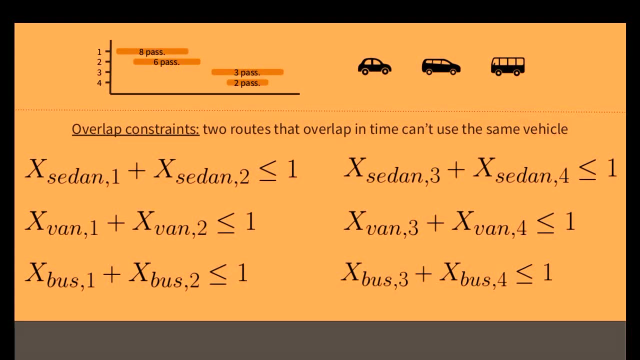 a bunch of equalities and it'll just turn them to two inequalities, So just wanted to get that out of the way. Great, Okay. So we have one last set of constraints here- Overlap constraints. These are actual inequalities. finally, 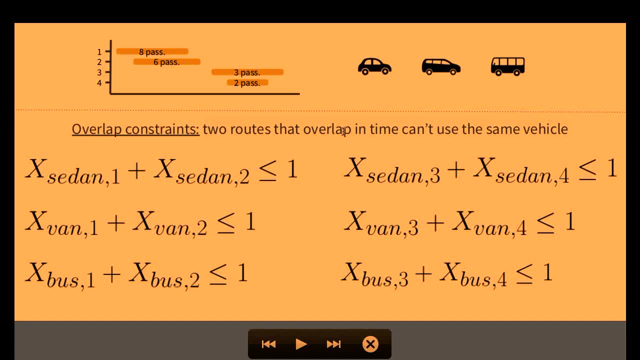 And these say that two routes that overlap in time cannot use the same vehicle, And so we have two pairs of routes here that overlap in time: one and two, and three and four. And so this cluster of three constraints is for routes one and two, and it's just saying that for every vehicle. 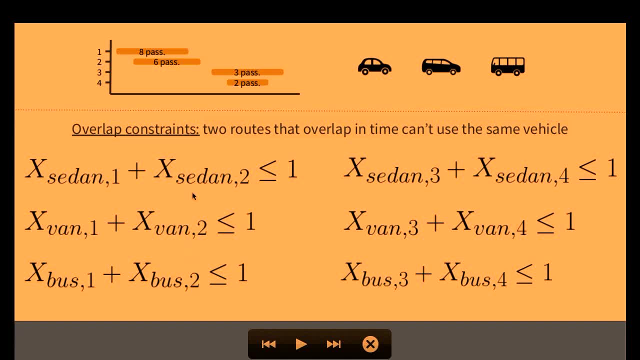 at a constraint that says you can't use this vehicle on both of these routes, And similarly for routes three and four. at a constraint that says you can't use for every vehicle. at a constraint that says you can't use this vehicle on both of these routes. 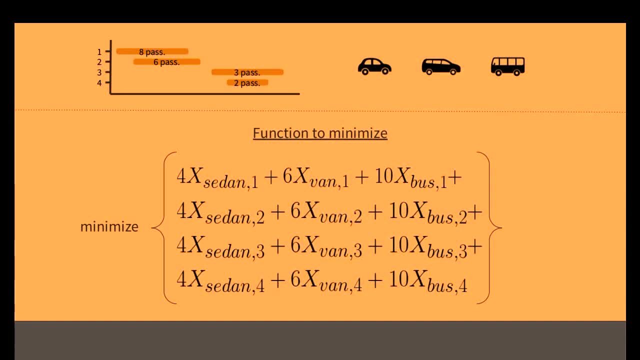 So we get six of these. Great, Now all that's left is the function to minimize, And this is the function we're going to minimize. Now, the constants here are the capacities of the vehicle, And this looks just like a big mess of variables and constants. 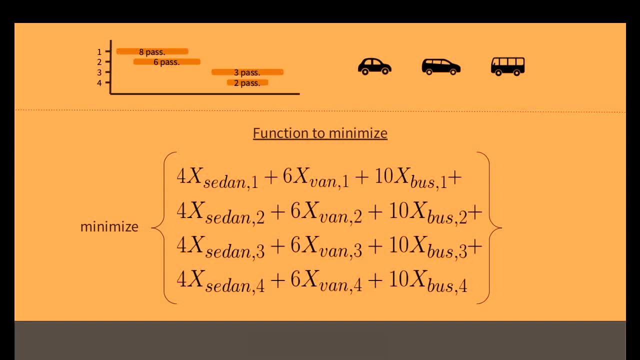 But if you stare at this for about 30 seconds- I'm not going to give you that 30 seconds right now- But if you stare at this for about 30 seconds, you'll see that each row in this very large sum is just the. 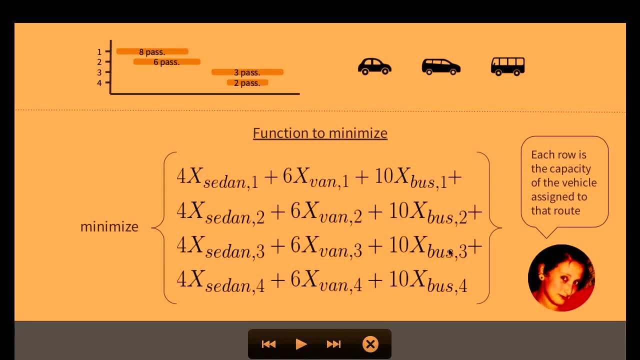 capacity of the vehicle that's assigned to that particular route. Right, This is what we're looking for. There's four rows, one for each route, And so this whole linear sum in total is just kind of the total aggregate capacity that we're deploying for all these routes. 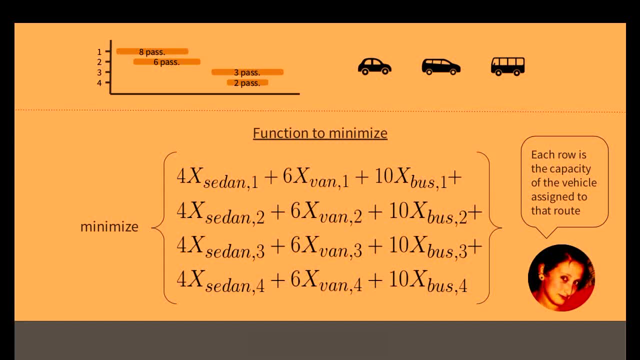 And again we want to minimize that because we want to avoid sending vehicles that are too big to server routes that don't need a vehicle that big. So we're just going to say, just add all these up and this will minimize the total capacity that we've deployed. 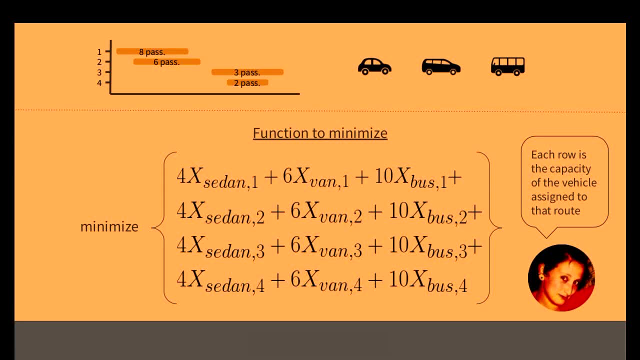 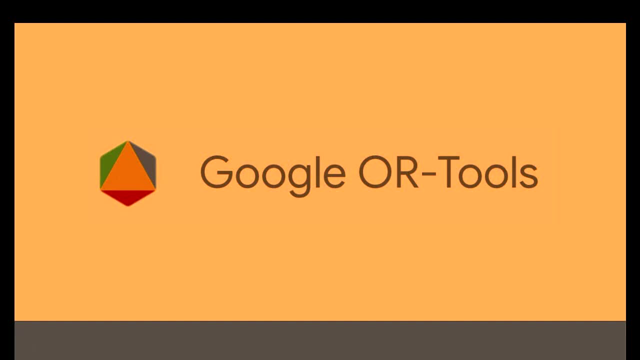 Okay, Great. So this is what our problem looks like, And this particular one is going to be, you know, a particular ILP-friendly mathematical form. So now let's switch over to a notebook and I can show you guys how to use OR tools to solve this problem. 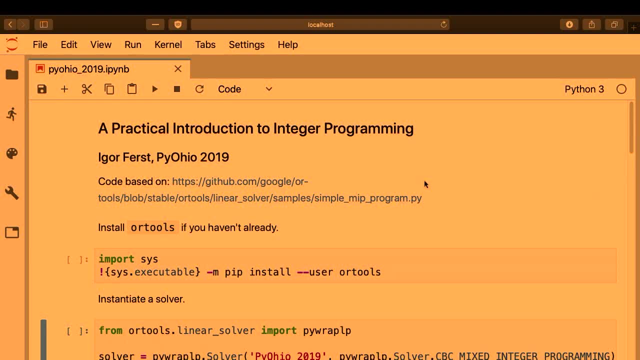 Can you see this? okay, Okay, Great. This stuff is going to be online. by the way, I'll have a link at the end of my presentation, So if you want to see the notebook and the slides, they'll be up on GitHub. 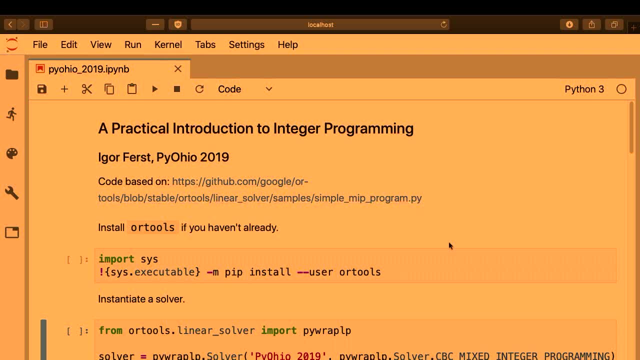 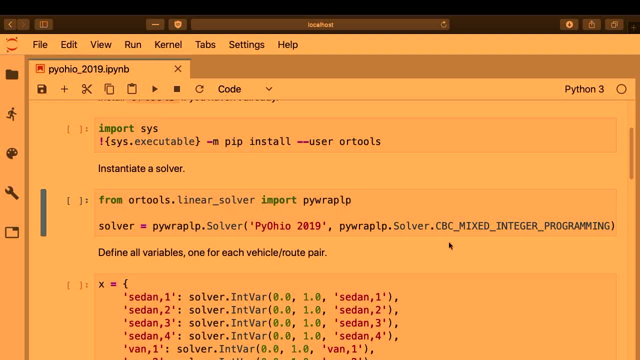 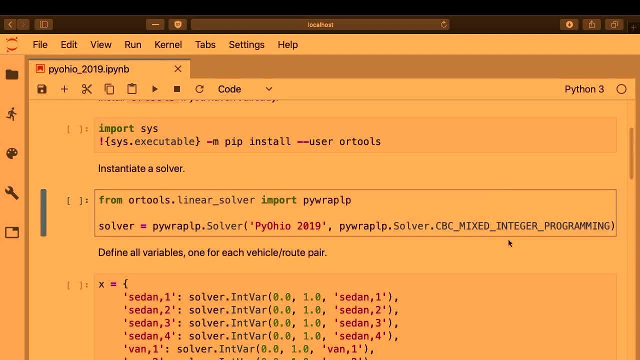 So using it is pretty straightforward And the fact that it's written in Python actually makes it highly usable. First thing you can do is, of course, I'll run this for you guys. You import OR tools and you tell it to instantiate a solver. 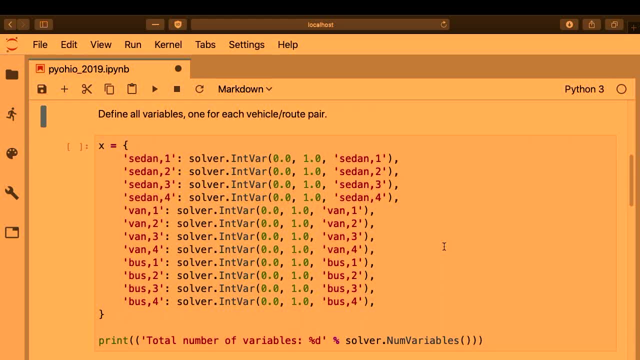 Great. First thing you've got to give that solver is your set of variables. And here we have 12 variables, one for each vehicle route pair. You just call solverintvar to define an integer value variable And we're going to say it must be between zero and one. 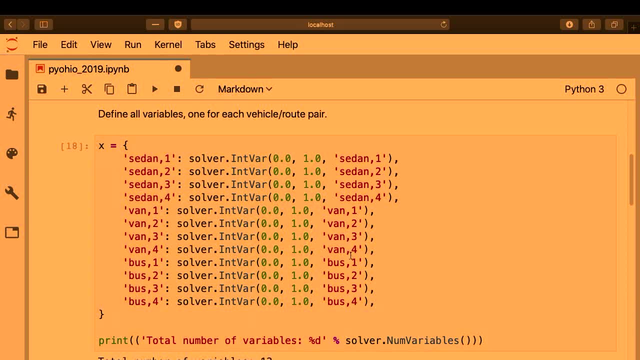 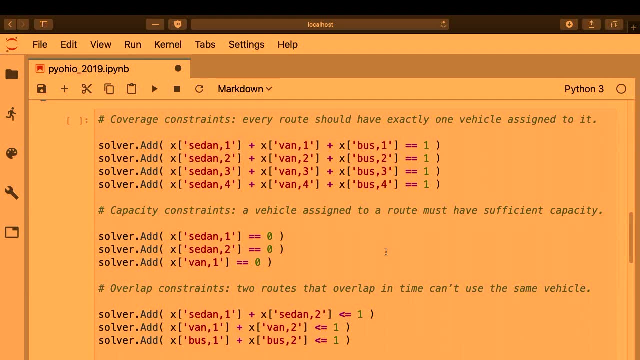 So, in other words, it has to be either zero or one. So we are going to instantiate these variables. Great, And now we just add all of our constraints to the solver. And this is really nice, because you can write this in Python. 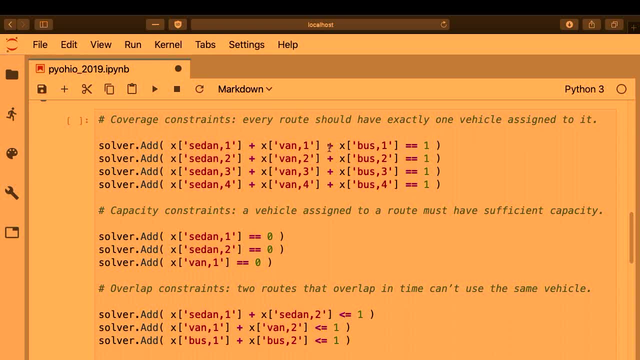 So you can write these expressions over your variables in a very human-readable form And then they'll evaluate to some magical object And you can pass it over to the solver And then they'll evaluate to some magical object And then you can pass that object to solveradd. 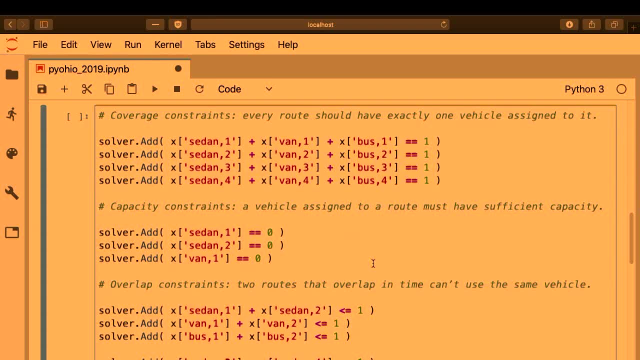 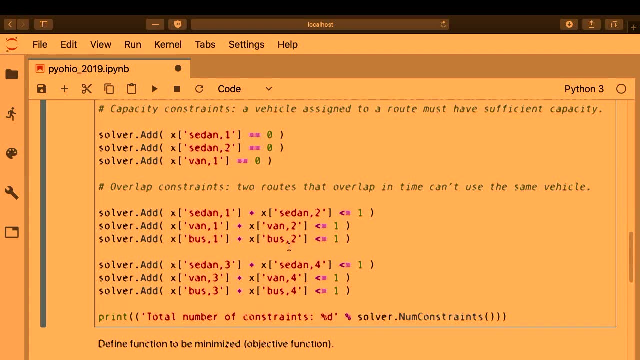 And this will just add all the constraints to the solver. So here we have our four coverage constraints, Here we have our three capacity constraints- exactly the ones that we just went over on the slides- And our six overlap constraints. So let's add all of them. 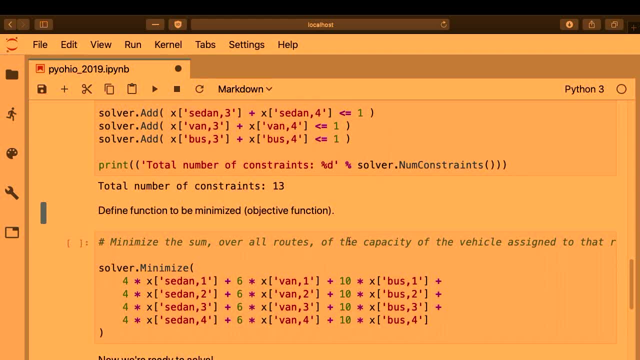 We have a total of 13 constraints- Great. And the last thing we need is the function to be minimized. And again, just like we saw on the slides, this is just going to be this very large sum over all the variables, Where we're multiplying by the capacities of the vehicles here. 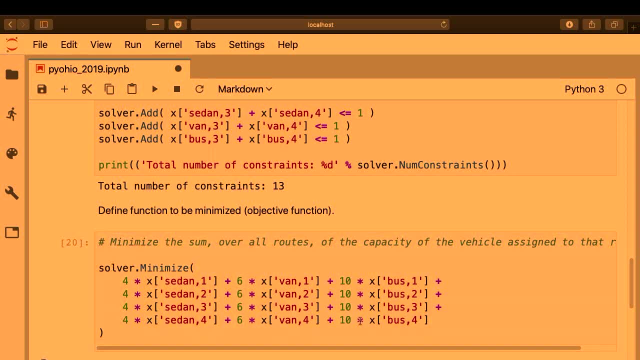 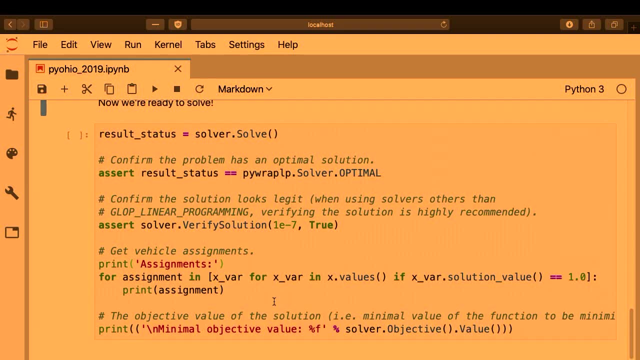 So we're going to add that as well. We're going to tell the solver to minimize this expression, this linear expression. Okay, And that's it. We've given it everything we've got, We're ready to solve, And so we just call solversolve. 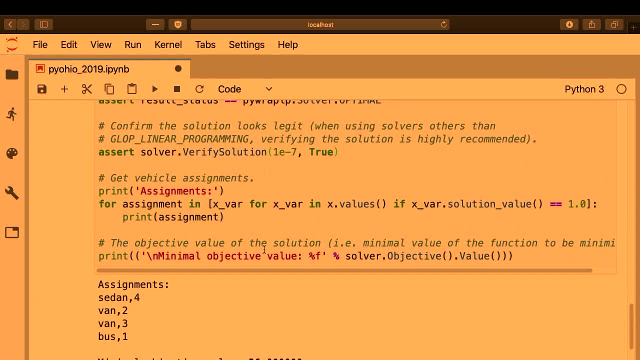 We verify that our assignment is optimal And then we print out all of the assignments. So we're just going to print out all the variables whose value is one, And this tells us that we're going to assign the bus to route one. We're going to assign the van. 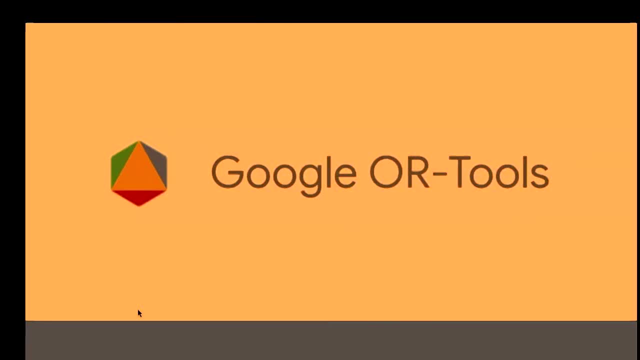 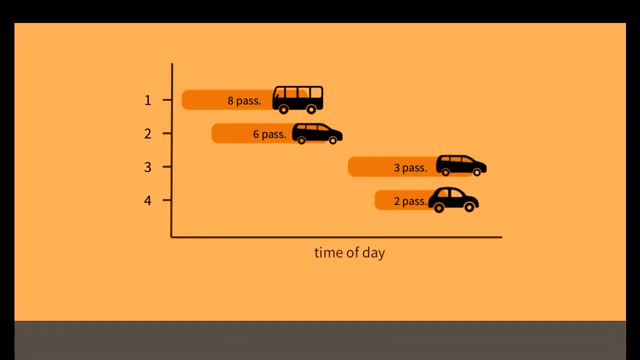 The van to routes two and three. We're going to assign the sedan to route four, So it looks like this. Which is you know? if you had kind of eyeballed this problem, you could probably figure this out. This is a pretty small scale problem. 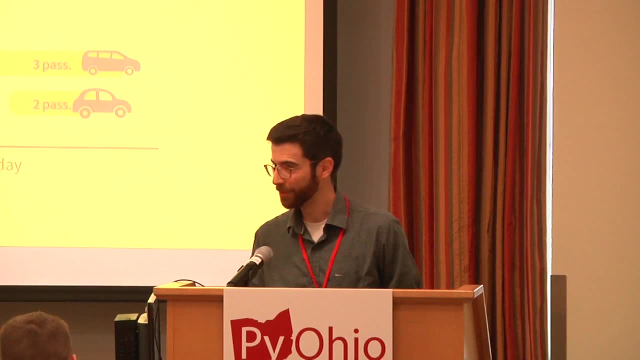 But of course the nice thing is that you can solve much bigger problems where the solution is a lot less obvious, And again the solution you get back is mathematically optimal. You know, given the formulation that you presented, is the best possible solution. 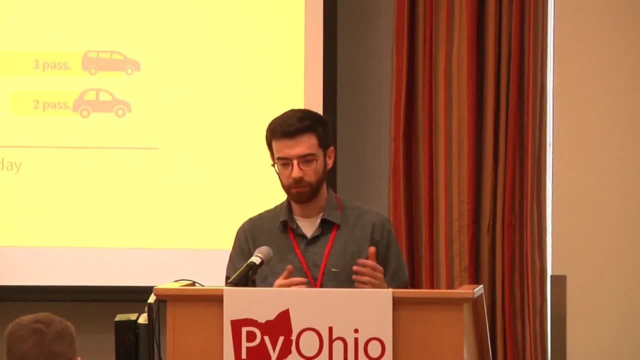 It's not always unique. There might be multiple solutions that are equally optimal, But it's guaranteed to give you one of those optimal solutions. if there happens to be more than one, Great Okay. So life is pretty good, right? You have this assignment problem. 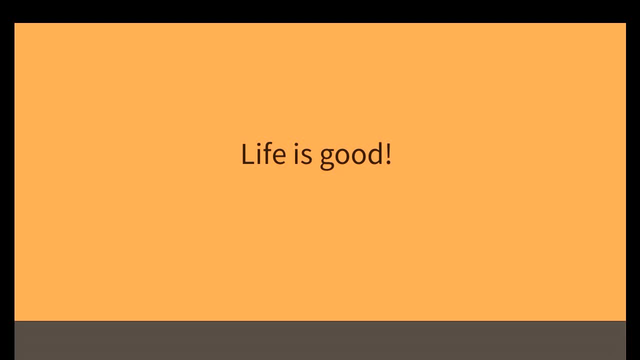 You can formulate it in this particular way: You just give it to a solver, Solver gives you an optimal assignment And everything's fantastic. Fortunately, life is not good. Life is hard and full of pain, And the problem here is that ILP is actually an NP-complete problem. 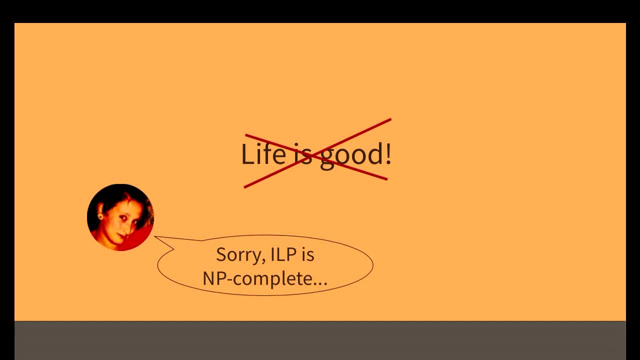 And if you guys remember your CS theory, that means it's a problem for which efficient algorithms probably just don't exist at all. And so, even though a lot of very smart people spend a lot of time and effort figuring out how to make ILP solvers as fast, 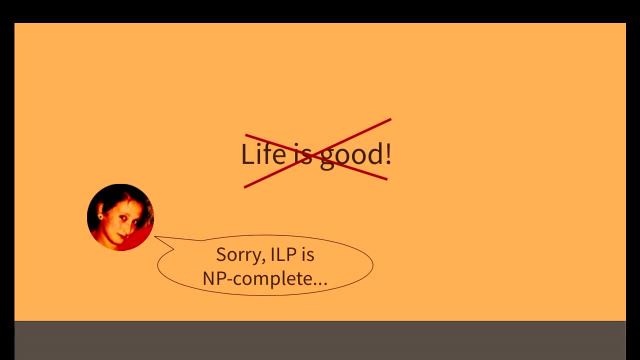 as possible. they're never really going to be that fast And all the ones that are available, both proprietary and open source, they kind of hit a wall even for moderately sized problems, because the problem they're trying to solve is fundamentally intractable. 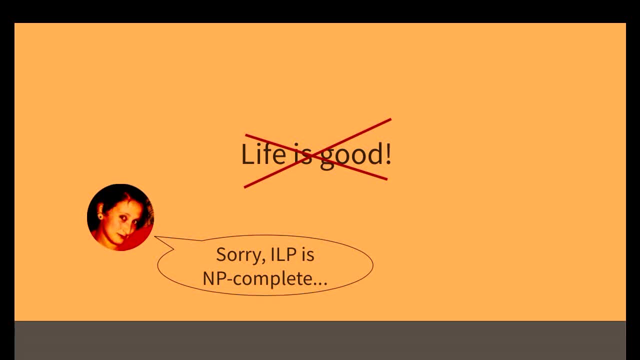 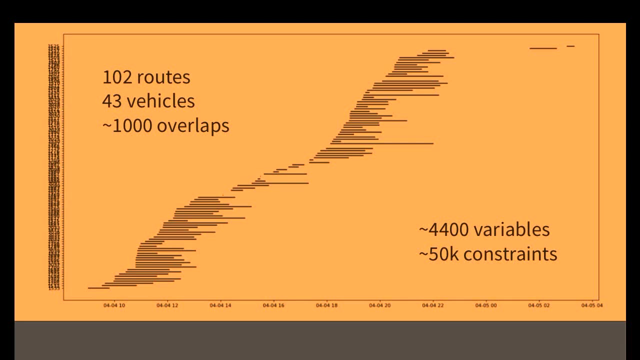 in a really formal sense. So we actually ran into this pretty quickly when we tried to solve the actual problem that was on our hands. This is a depiction of the kind of fleet assignment problem that we were dealing with. This is one day in the operation of this private shuttle service. 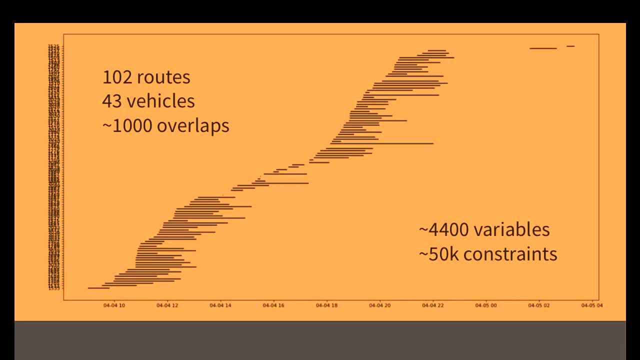 And here we're talking about 102 routes, a fleet of 43 vehicles and about 1,000 pairs of overlapping routes, And this results, if you just kind of like go through the naive process that we just went through, in almost 50,000 constraints. 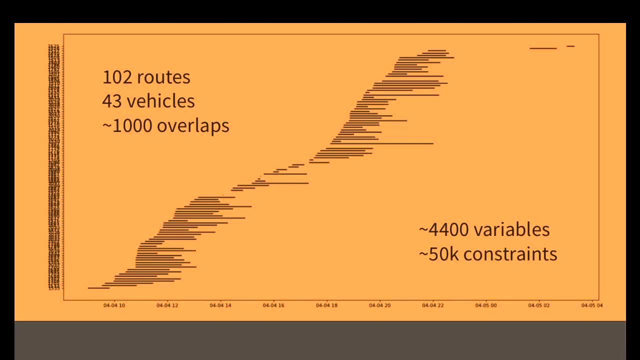 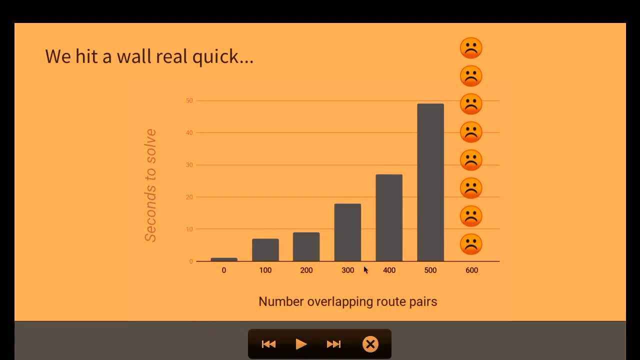 Which is large for an ILP solver, And so what happens here is that we hit a wall actually really quickly. If you. this is a little chart that shows how fast it took to solve subproblems. They just restricted the number of overlapping route pairs. 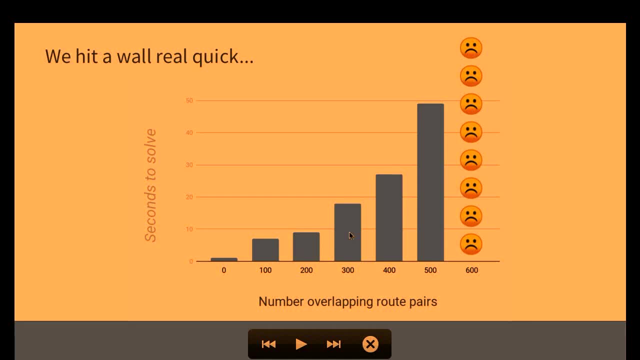 So you can see between 100 and 500 overlapping route pairs. you know there's an increase that looks uncomfortably exponential And our problem again had about 1,000 overlapping route pairs And then between 500 and 600, there's just some kind. 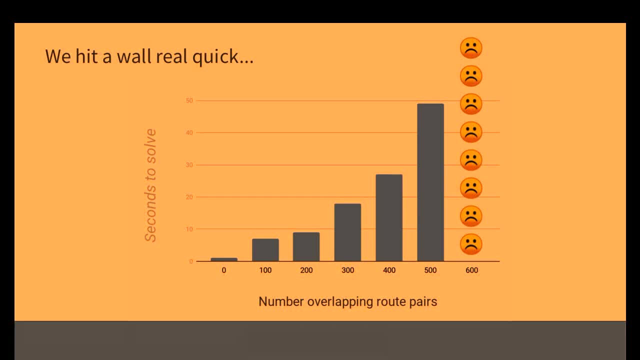 of weird phase transition where I just kind of stopped waiting after 90 minutes and just didn't finish. And this is what happens all the time. This is just the name of the game. when you're working with ILP, You know you're using the solver in a black box fashion. 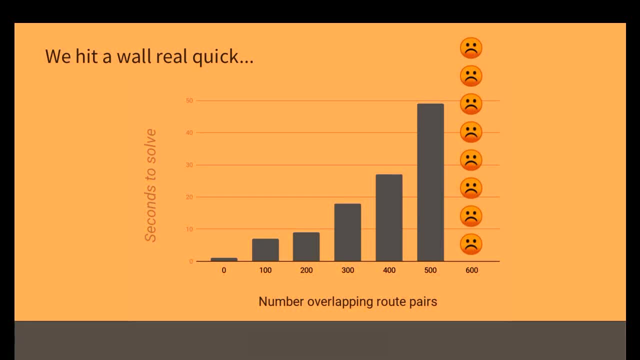 The solver is trying to solve a problem that's empty, complete. You know, the increase in the amount of time it takes to solve a problem goes up very quickly, And then sometimes you just hit a wall where it's just not going to end in any reasonable amount of time. 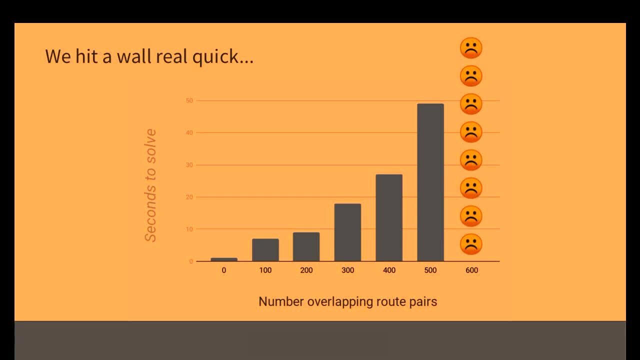 So what do you do? What do you do in this situation? Well, what you have to do is be very, very clever about exploiting the structure of the specific problem that you're trying to solve. There's only so far you can get by, just you know. 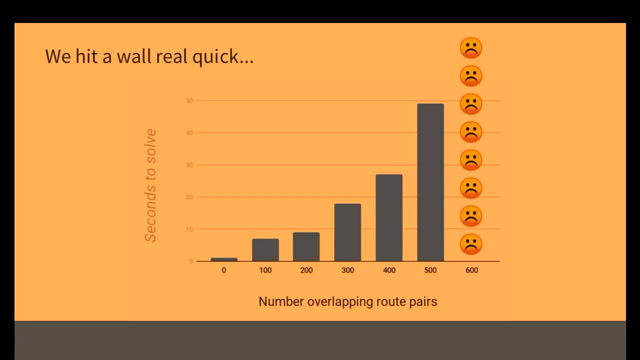 kind of like performing a general transformation and feeding it into a general purpose solver. And this is something that happens all the time in ILP- And I'll have another great example of that in a few slides- And it's also something that we had to do in order to be able. 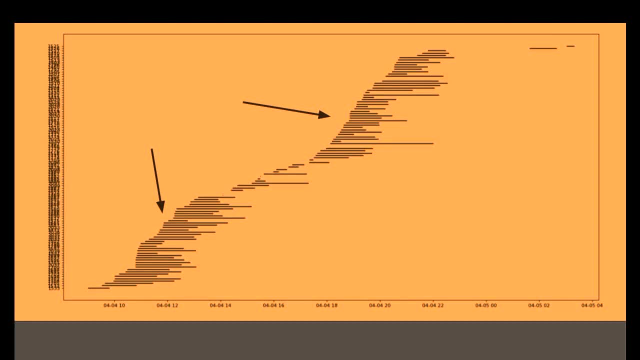 to solve this problem at all, And so one thing we noticed is that the distribution of these routes is pretty bimodal. This is a shuttle service that generally just takes people to and from work, So there's a lot of trips in the morning here going to work. 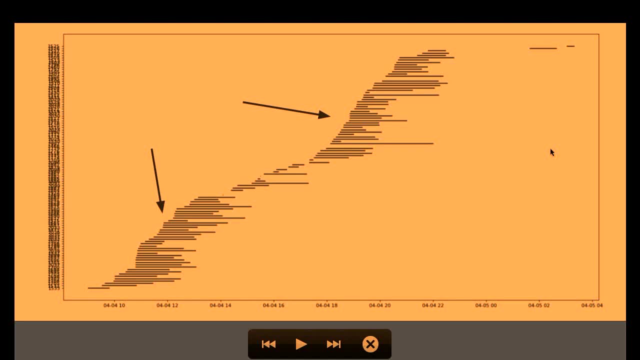 a lot of trips in the evening going home from work And so for almost all days it's actually pretty easy to just kind of like split the day in half, solve the individual subproblems for the first part and the second part of the day. 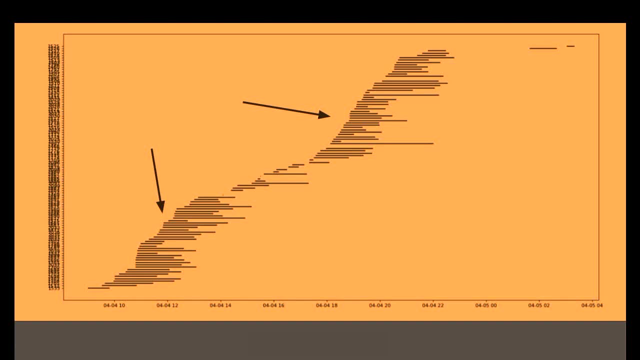 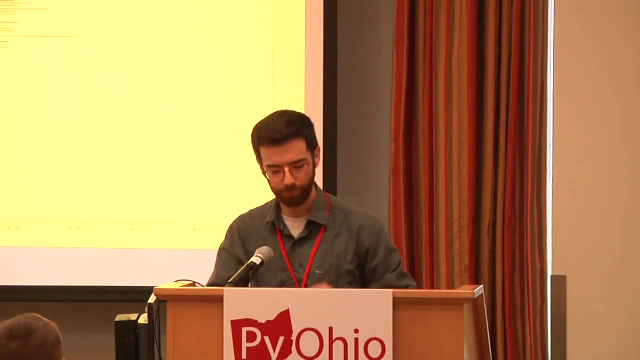 and then combine those into a solution for the entire day. And that's straightforward because you know it's pretty bimodal. There isn't a lot of routes that just you know span those two parts of the day, So that made it feasible to just kind of solve the subproblems. 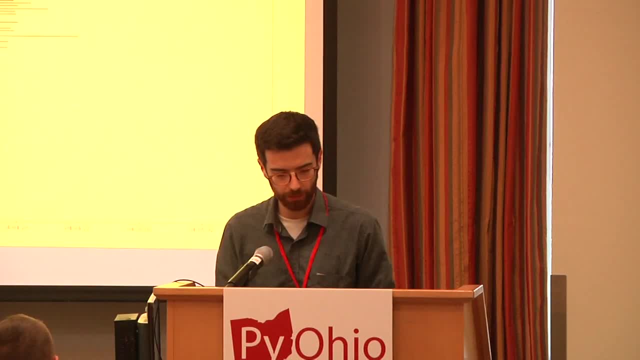 which you know just took a few minutes, and then combine them And we were in a good place. And again, this is something that happens all the time in ILP And there's also, like I mentioned at the beginning of the talk, a great illustration of the fact that you know. 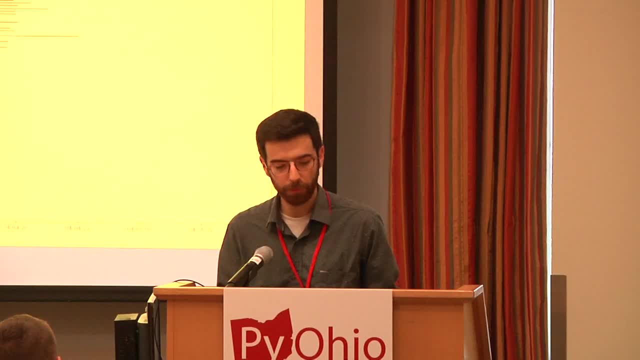 when you're solving real-world data problems, you know you have to pay very close attention to the structure of your problem, because general tools really only take you so far. So let me give you another example. that is really great. This is one of Rachel's favorite papers. 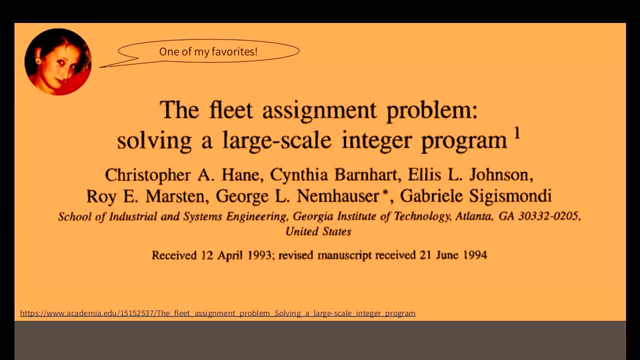 This is a paper about a fleet assignment problem, but it's actually an airline fleet assignment problem. So some folks at Georgia Tech were asked by an airline- We don't know- they don't say who it is, but it's probably Delta- just because they're also. 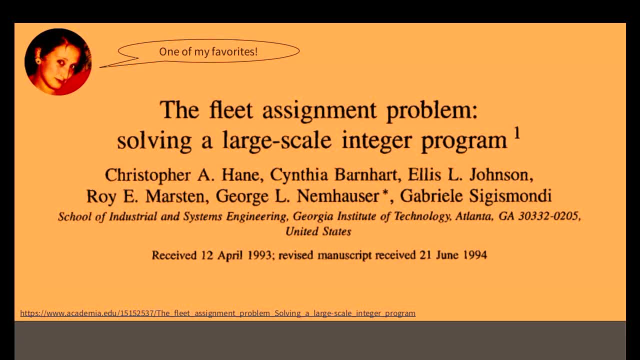 in Atlanta. So some airline, probably Delta, asked them to solve this, this vehicle fleet assignment problem for their planes. right, They just want to make sure that they are assigning their planes to their routes as optimally as possible. And this is a really interesting paper, because these folks 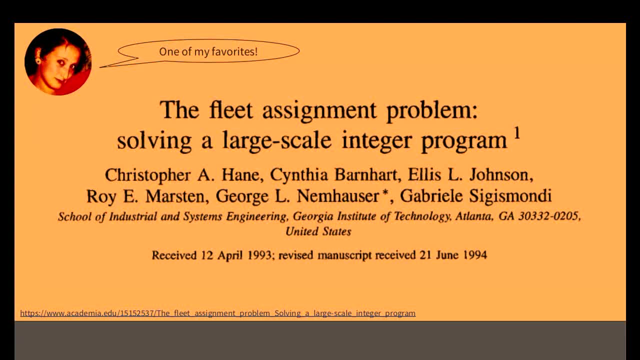 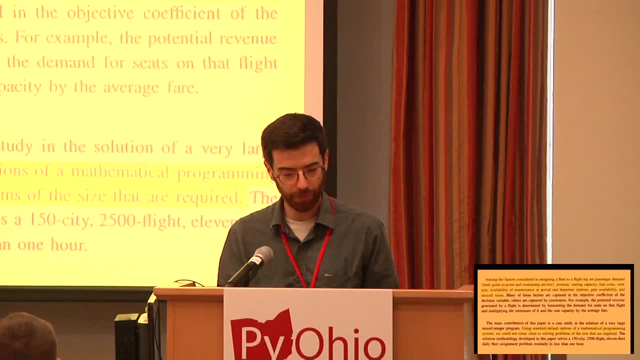 at Georgia Tech. they want to make the problem as realistic as possible. They want to make it very useful for their client, And so they put in all of the relevant constraints- And there's a lot of these. So the airline cares about constraints around passenger. 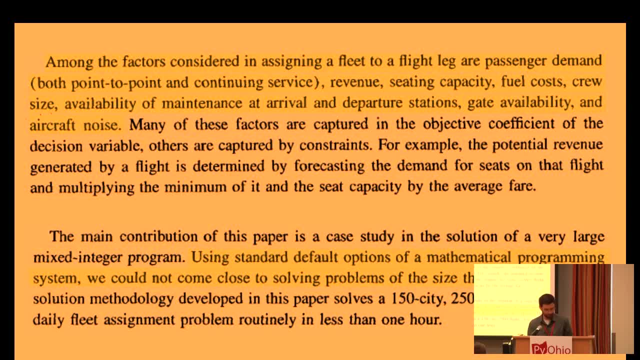 and demand revenue, seating capacity, fuel costs, crew size, availability of maintenance. You know they want this to be as realistic as possible, which results in tons of constraints, tons of really interesting constraints. And they say in the paper here: using standard default options. 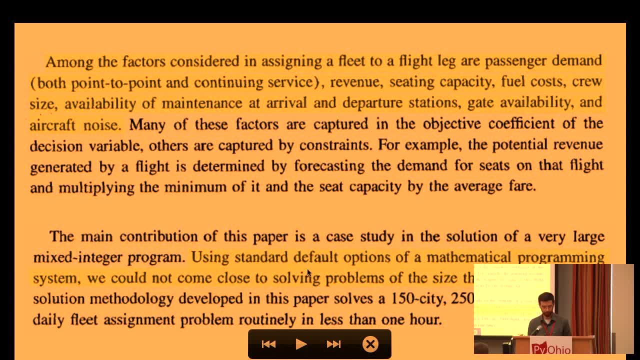 of a mathematical programming system. we cannot come close to solving problems of the size that are required. They're working with 150 city, 2,500 flight assignment problem, which is like this isn't big data, right? I mean, you know we're talking about like hundreds. 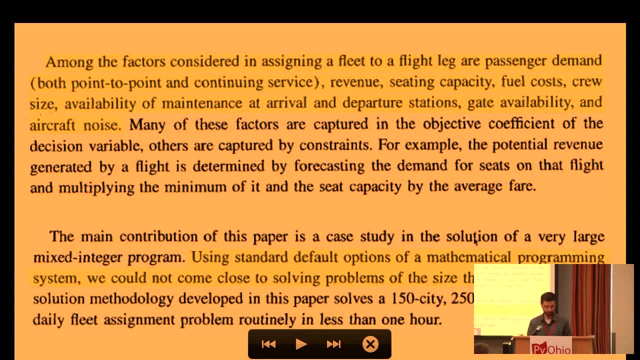 and thousands of things right, But for ILP this is a very big deal, right, And so just using default options, they couldn't even come close to solving a problem of this size, And so this whole paper is 20 pages, all about how they very 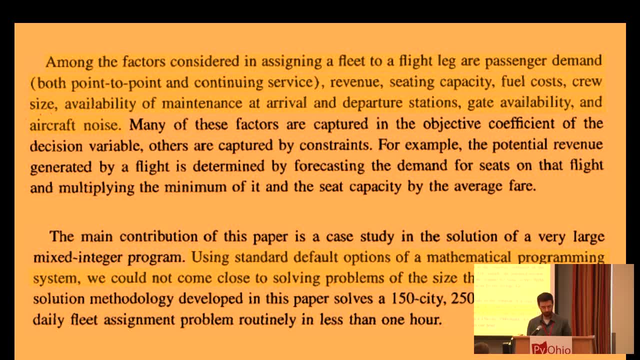 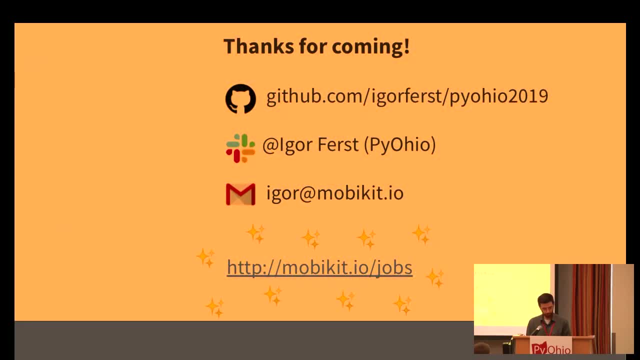 very cleverly exploited the structure of the specific problem they were trying to solve in order to make this tractable, And it's super interesting. if you're into this kind of thing, Great. So that's it. All the stuff from this talk is on GitHub- the slides: 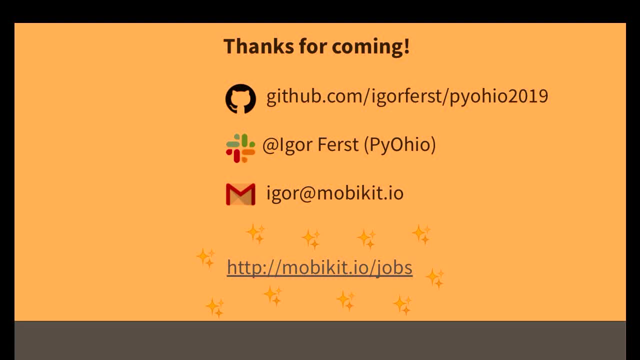 and the notebook if you're interested in that. If you have any more questions, we might have a few minutes here. Feel free to catch me in person. I'm on the PyOhio Slack. You can reach out to me there. You can email me.